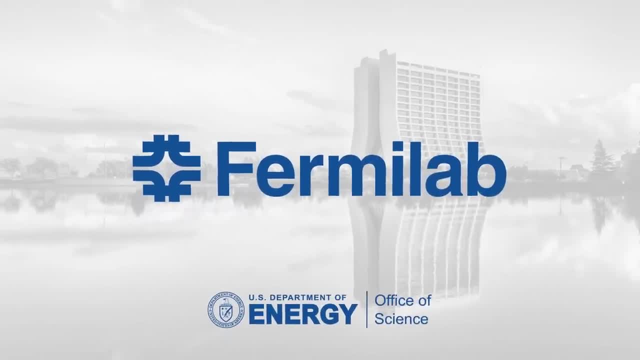 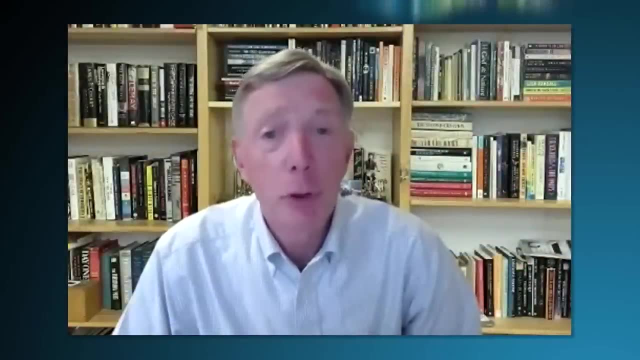 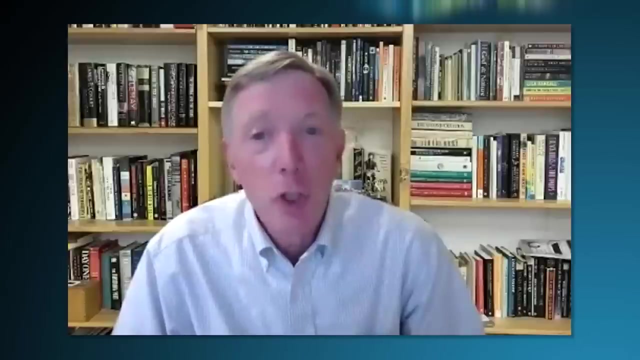 Hello, I'm Dr Tom Carter from the College of DuPage and I'd like to welcome you to another InfermiLab series of talks on physics and science. It's not often that you find a scientist that has the unique combination of work in theoretical particle physics, film and television. 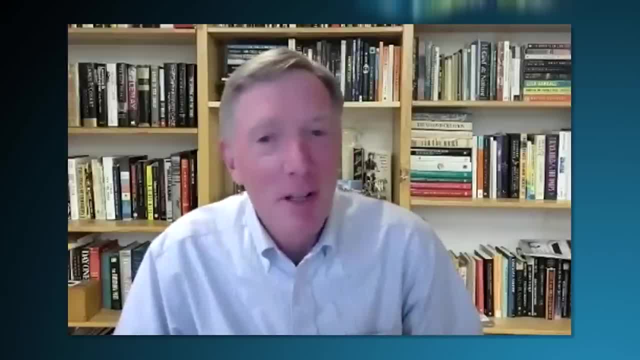 Our speaker tonight, David Kaplan, has that combination. Dr Kaplan received his undergraduate degree from the University of California at Berkeley and his PhD from the University of Washington. He held postdoctoral positions at the University of Chicago Argonne National Lab and the Stanford Linear Accelerator. He joined the faculty of Johns. 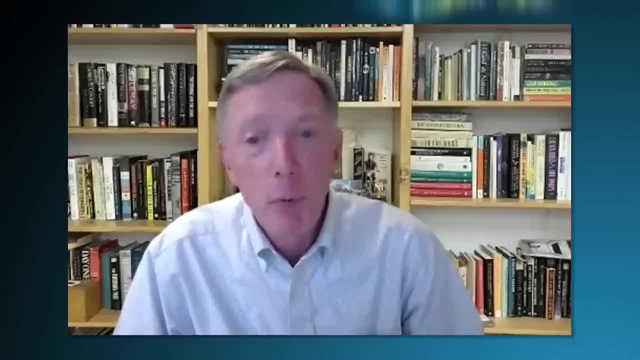 Hopkins University in 2002.. His primary research interest is in physics beyond the standard model and in the field of physics. He's a professor at the University of Washington and he's a particular focus on the Higgs mechanism and potentially related physics such as supersymmetry. 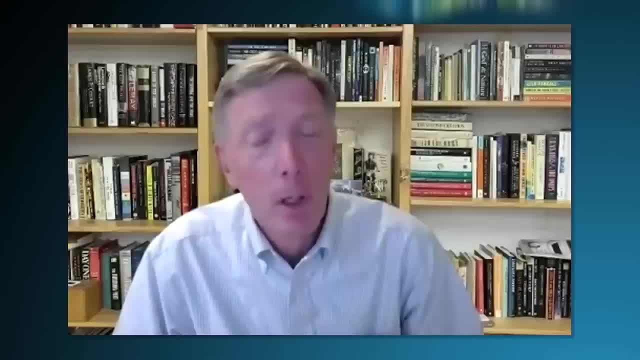 new forces, extra dimensions and dark matter. An American Physical Society fellow, Dr Kaplan, was also awarded the National Academy of Sciences Kavli Frontiers of Science Fellowship and an Alfred P Sloan Fellowship And he was awarded an outstanding. he was named an Outstanding Junior. 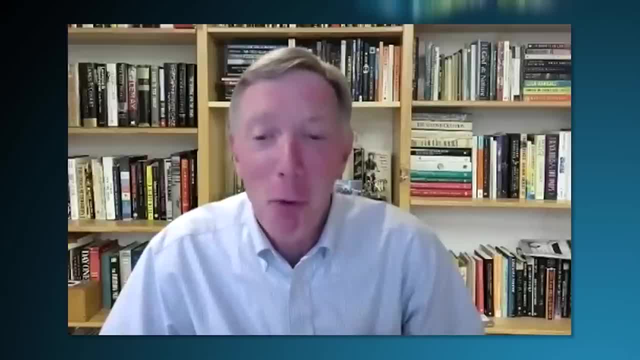 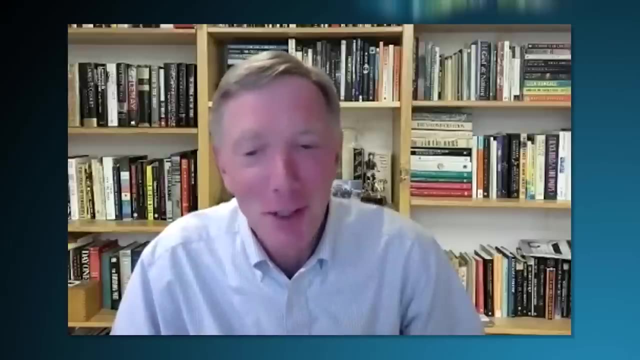 Investigator by the Department of Energy. As I mentioned before, Dr Kaplan has also worked in films, having created and produced the documentary Particle Fever, which won the Alfred DuPont Columbia University Award. To top it all off, he co-hosted. 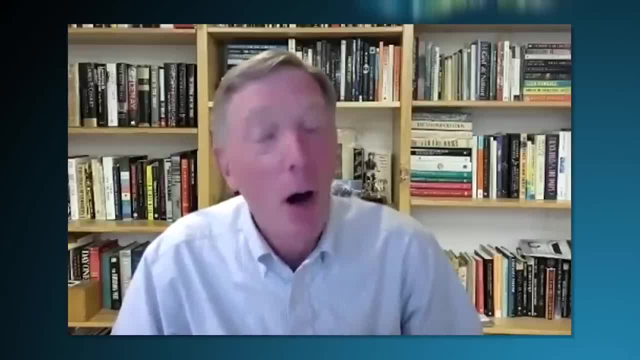 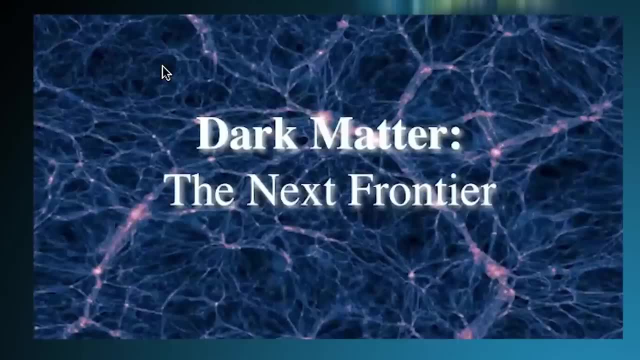 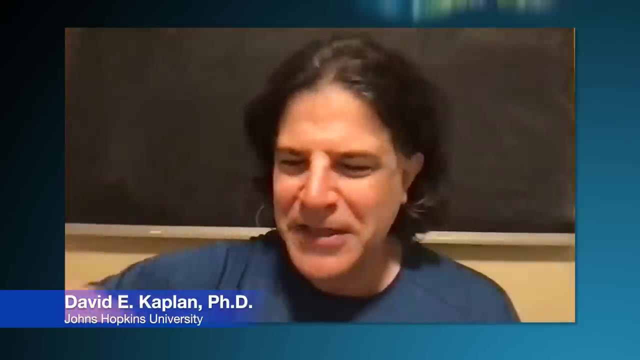 season three of the National Geographic's Unknown Universe television documentary series. Let me introduce Dr David Kaplan. Thanks, Tom, Hi everybody. Hi everybody. Sorry to not be all together in the same room, but it's great to be able to talk to everybody. 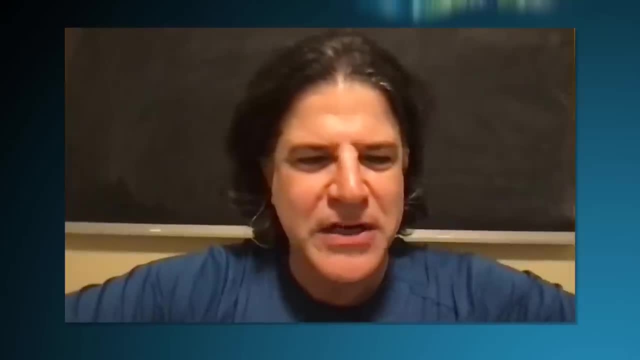 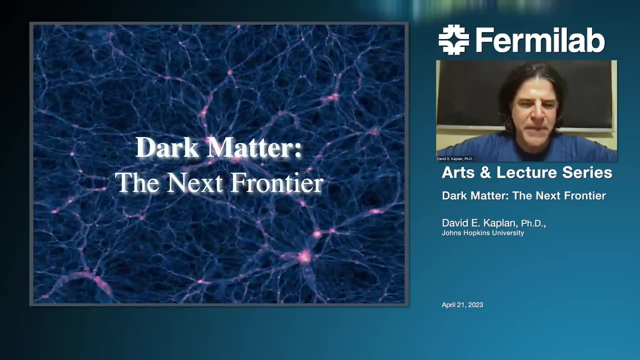 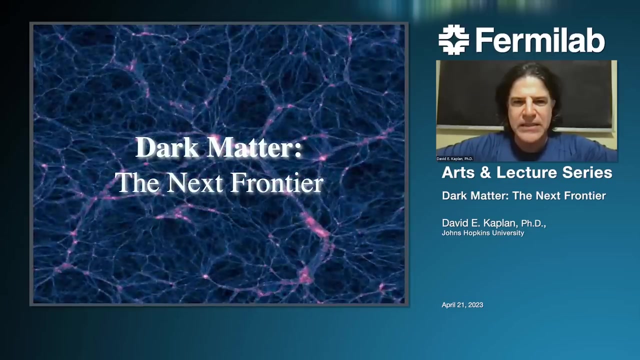 and tell you what I'm excited about right now. This talk is going to be about dark matter. Let me share my screen. Dark matter is one of a number of things I think about and work on, and it is something that scientists from many different disciplines actually think. 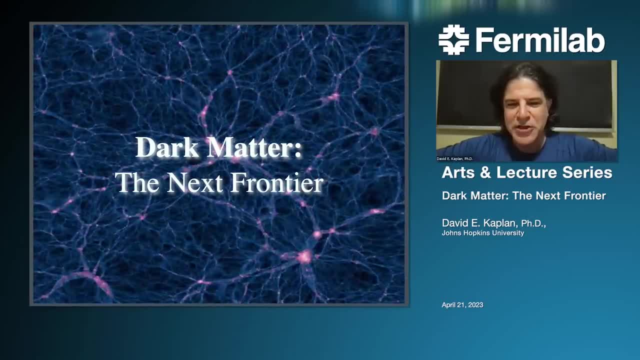 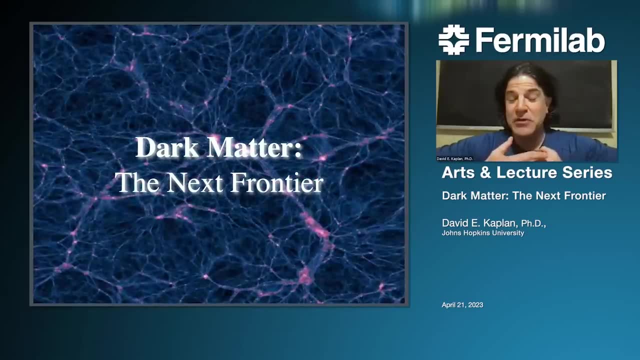 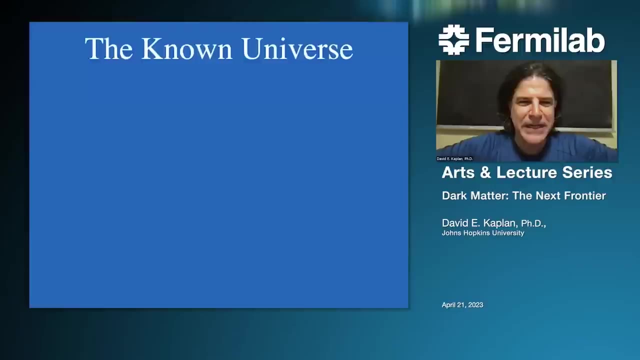 about from astronomy and astrophysics to cosmology, to particle physics. So I'm giving you the particle physics point of view, And one of my responsibilities as being a particle physicist is to figure out what this stuff is. So let's begin, Before we talk about something unknown. 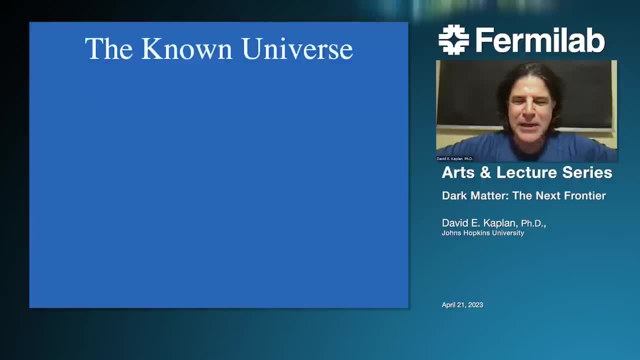 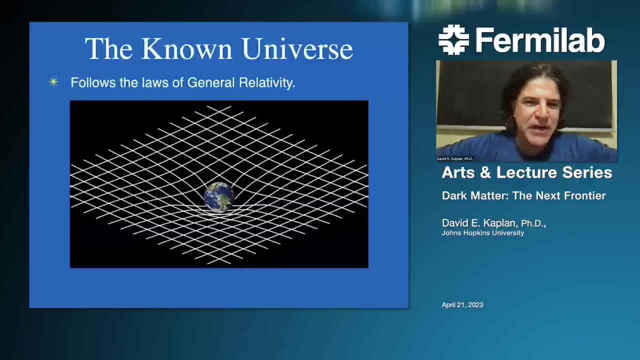 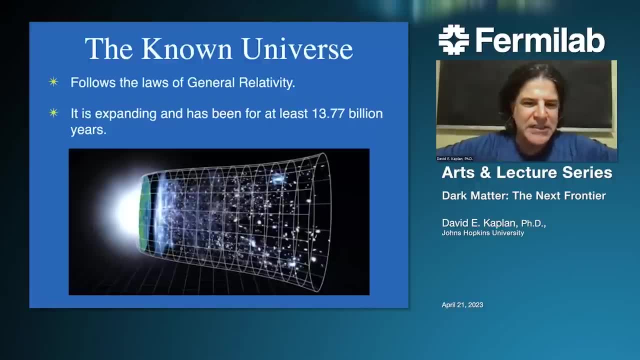 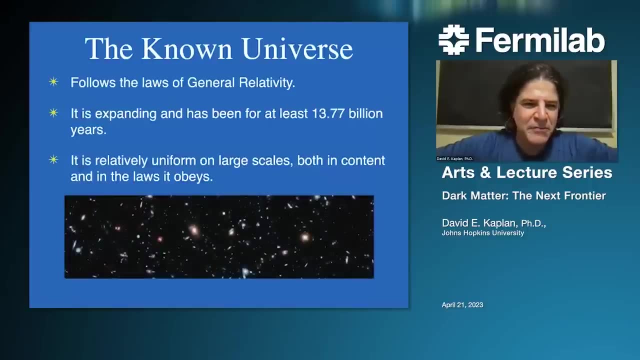 Okay, Okay, Okay, Okay, Okay, Okay Okay. The universe and everything in it seems to follow the laws of general relativity, And the universe itself is expanding, and has been expanding for at least 13.77 billion years. It's relatively uniform on the largest scales. 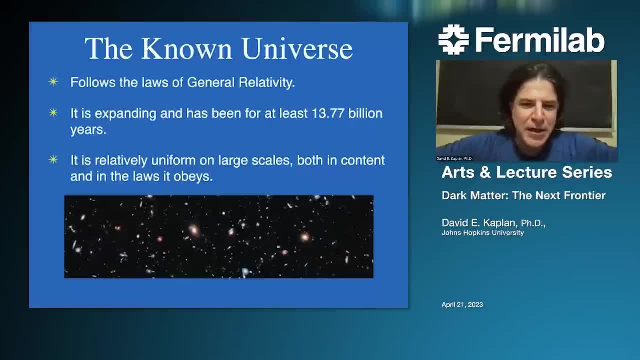 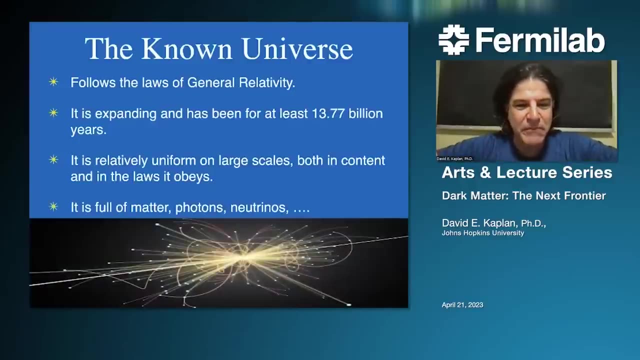 There's stars and galaxies and lumpy things in it, But it is over the entire universe that we see quite evenly distributed, And that not only includes the stuff but the laws that govern that stuff seems to be the same everywhere. And what is it full of? It's full of galaxies, and 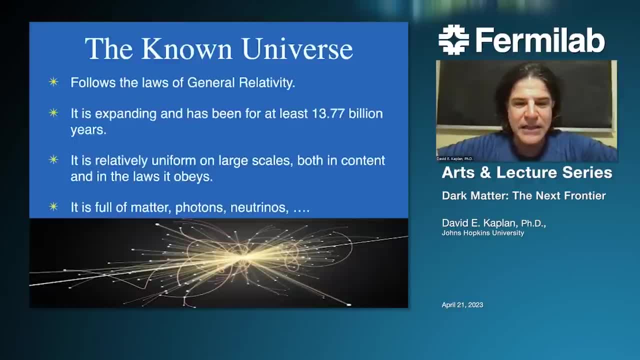 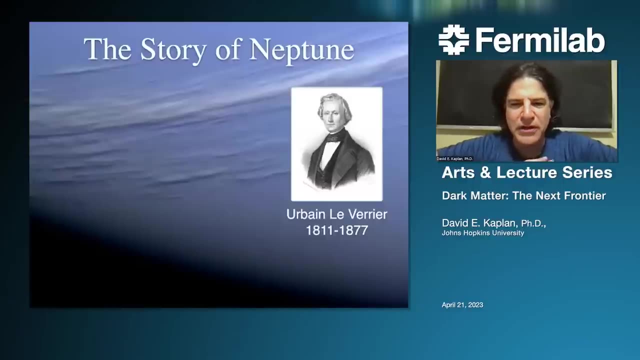 stars, but at the fundamental level, it's full of matter and the things that make up matter and photons, which are what we name particles of light and neutrinos. So, in order to talk about dark matter, I want to talk about it in a historical analogy. 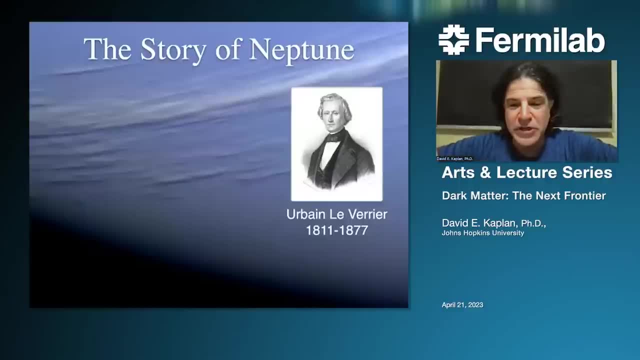 I want to talk about this story of Neptune. which is responsible? its discovery is responsible by Urbain Le Verrier. So the story goes in late 1845, Le Verrier found that Uranus's orbit was not following Newton's laws precisely, And it was enormous amount of water. 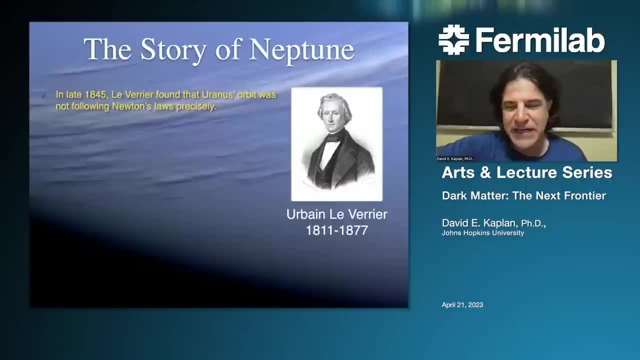 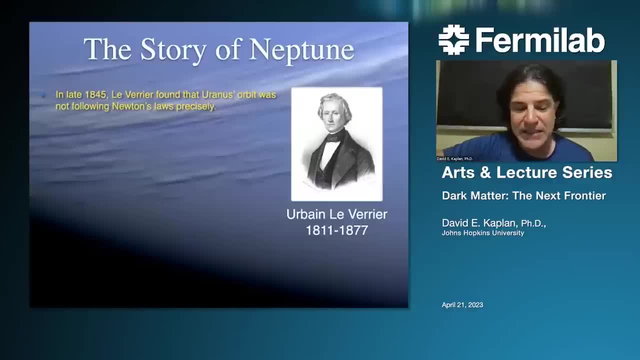 to the gravity of the sun, but all the other planets in the solar system. But through incredibly careful and complicated calculations, he was able to verify that something was wrong with this orbit, And so, in fact, he guessed that there's another planet out there whose orbit is perhaps a little. 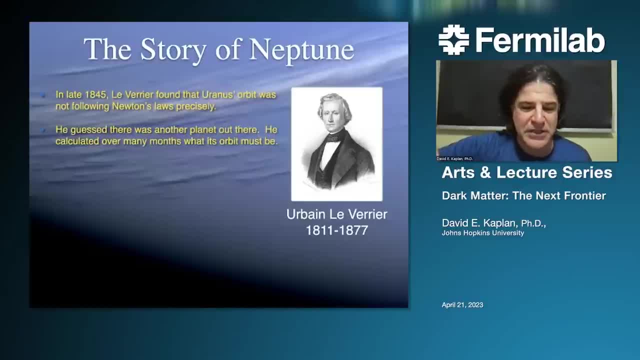 farther than Uranus, but close enough to influence Uranus's orbit. He made this calculation over many months to figure out what the orbit of that new planet should be, wrote his prediction in a letter that was sent to astronomers at a major telescope in Berlin. And on September 23rd 1846, the day 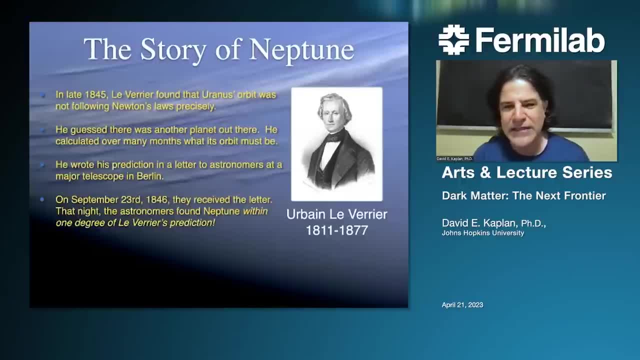 they received the letter. that night the astronomers went and looked in the location that Le Verrier suggested And, within one degree of the prediction, found a new planet, Neptune. So we often say Le Verrier had discovered a planet with the point of his pen. What he did was take the known laws of physics. 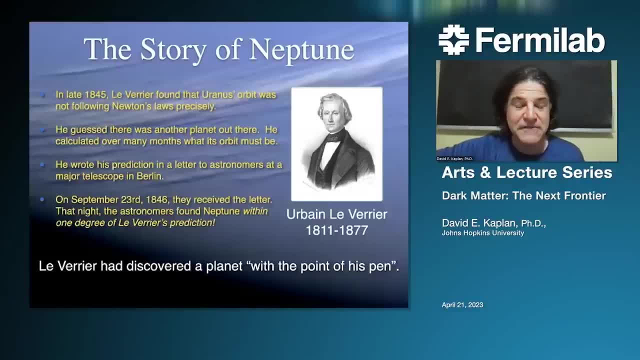 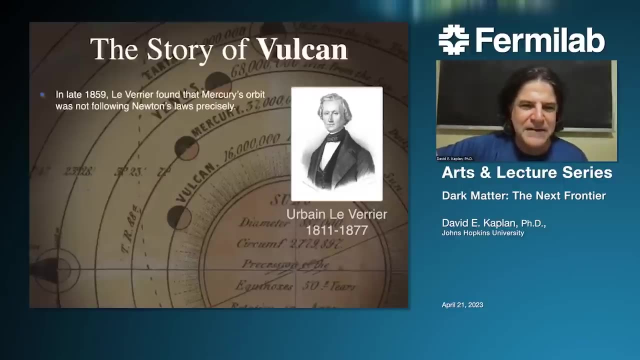 the laws of gravity do very precise calculations and find a deviation, and predicted something else within those laws was having an effect. Super confident after this amazing, amazing discovery in late 1859, working out Mercury's orbit, which is harder to detect experimentally. because it's so close to the sun, So it's actually harder to see Mercury for the telescopes. at the time, Le Verrier found again that Mercury's orbit was not following Newton's laws, precisely after taking into account the gravitational forces from all the other planets nearby. So he announced there must be a new planet, which he named Vulcan and estimated the orbit that Vulcan should take Vulcan even harder to see because Vulcan's orbit was predicted to be inside the orbit of Mercury and therefore even closer to the sun. In December of that year, French astronomer wrote to Le Verrier with the discovery of a planet, but it was not confirmed and decades of controversy and contradictory data ensued. 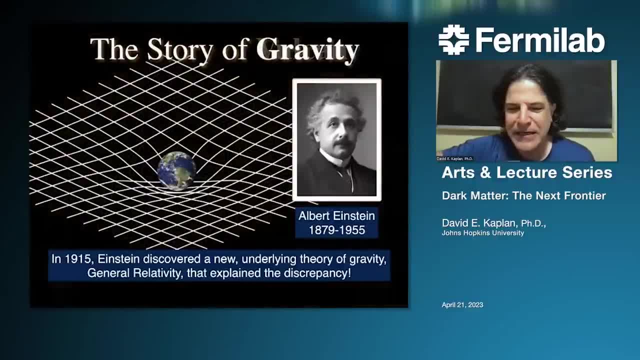 Many, many years later, the scientists at the University of Paris, at the University of Paris, had discovered a new planet which was called the Sun. Many, many years later, Albert Einstein- in 1915, discovered a new underlying theory of gravity called general relativity, and that explained the discrepancy. It required a new law of nature to explain the dynamics, and this was a totally different way, but using the same calculational tools, new physics was discovered. 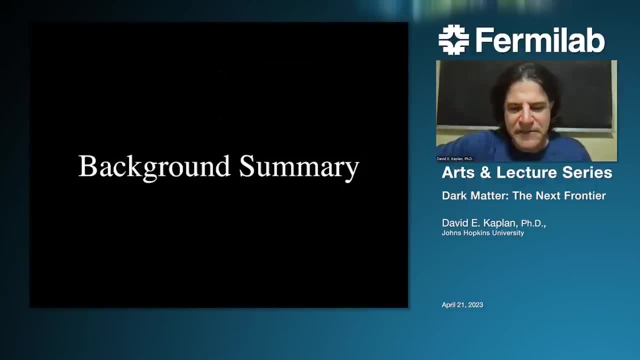 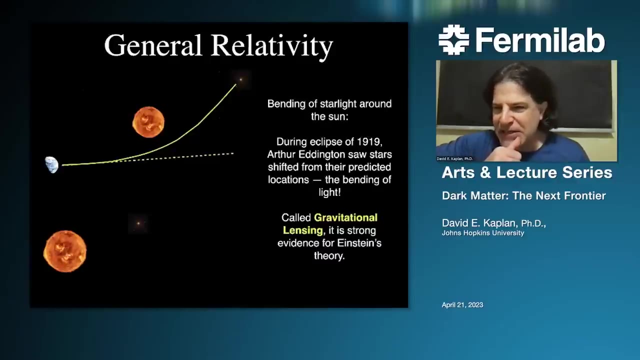 All right, First I'm going to give you a little bit of a physics background and or cosmology background, and then we will dive into the mystery of what dark matter is or does and might be. First of all, general relativity has some just amazing properties, and one of the properties is the fact that matter which has, say, a gravitational field around it, bends light, So it doesn't just attract other matter, but it attracts anything else. 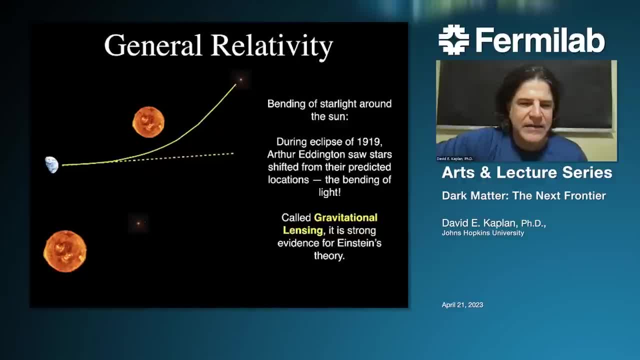 It attracts anything that contains energy, And since general relativity predicted this, Arthur Eddington led one of two expeditions for the 1919 solar eclipse And therefore was able to look at stars that were near by the Sun, but now very carefully with photographic plates, and determine whether the light bent and discovered it. 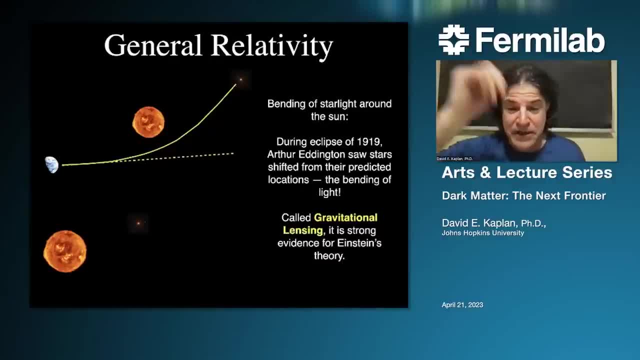 And therefore was able to look at stars that were nearby the Sun, but now very carefully with photographic plates and determine whether the light bent and discovered it. This discovery was a discovery of what we call gravitational lensing, and the whole point is that if you see some distant object but there's a close-by object with gravitational force nearby and sort of in the line of sight, then that beam of light coming from the distant object will bend. 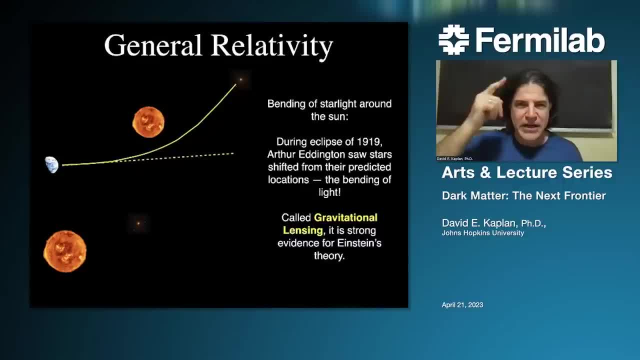 And your eyes will perceive it as our brain interprets. light appearing on our optical nerve is in a straight line away and directly towards the point that you see it, So as a star, let's say below, is at a specific location. if a massive body moves nearby, along the line of sight, then its apparent location will deviate from where it actually is. 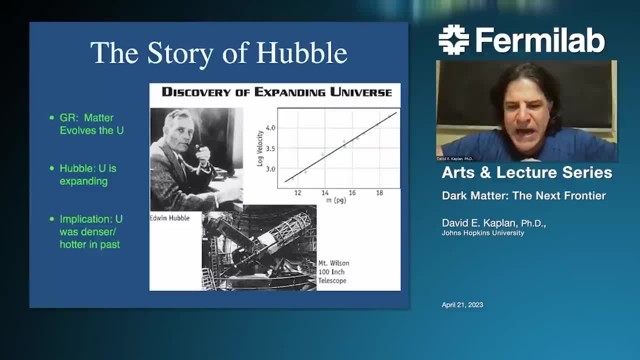 The other thing general relativity predicted is that matter could be described as warping: the universe, the entire universe, because the entire universe contains matter, And so, in fact, general relativity predicts that the universe is not static. it should be doing something, its shape should be changing. And Hubble, only a couple years after the Eddington discovery, discovered evidence that the universe was expanding. The Method was to look at distant galaxies- and different galaxies were already a new thing- and see not only that they are moving away from us, which is what he discovered, but that the farther they are, the faster they're moving away. 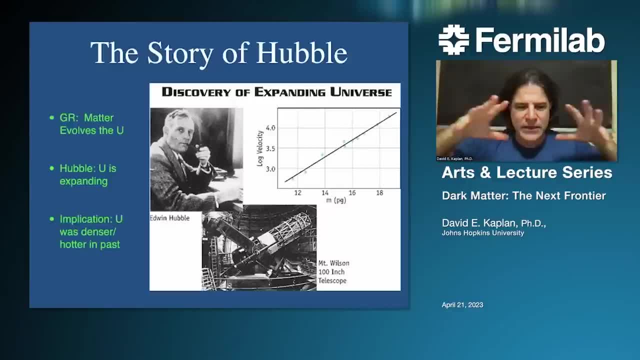 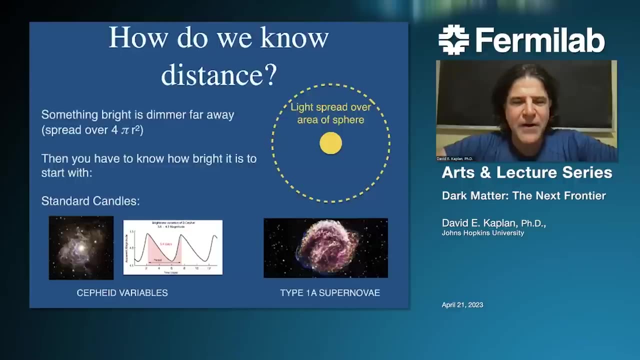 And that on a whole, taken, broadly, looks like the universe is expanding And that's an implication that if the universe is expanding now, it must have been smaller, denser Or even hotter in the past. Now it's very easy to say that Hubble looked, saw some galaxies, saw that the farther they were, the faster they're moving. 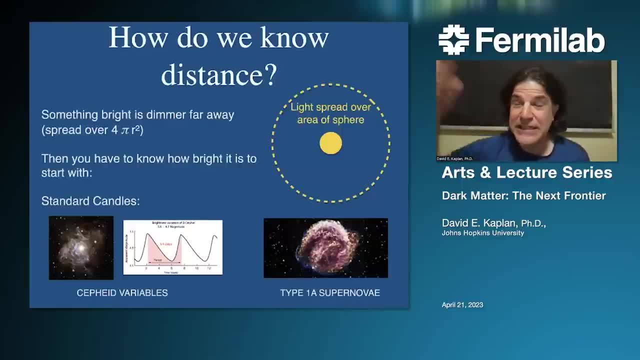 But how do we actually measure distance? You see a dot in the sky. how far away is it? It is harder than you might think to measure distances in the universe, Something which is bright, of course, but far away is much dimmer. 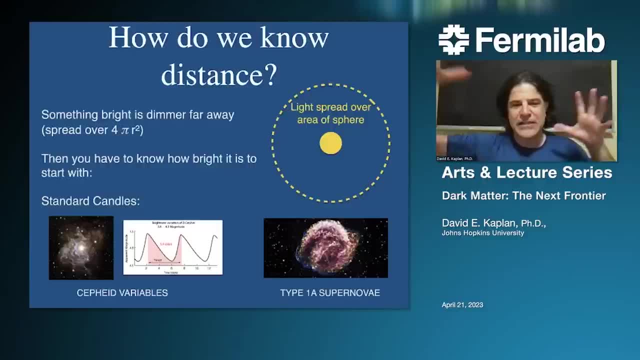 Because The light spreads out over an area, let's say 4 pi r squared, or the surface of a sphere, And so the farther you are from the point, the less of the light you collect in your eye or in your telescope. 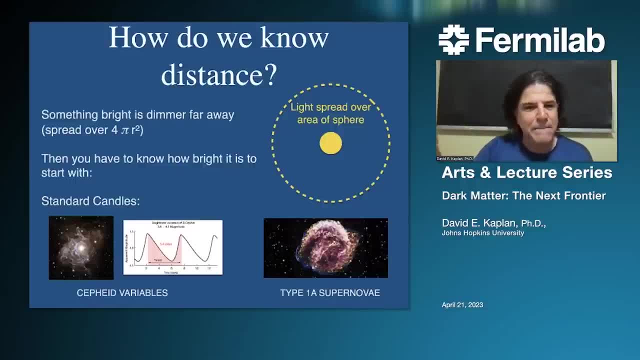 So you could determine how far it is by how dim it is, but only if you know how bright it was in the first place, And there are many different types of stars and galaxies with different brightnesses, But we have found over the years so-called standard candles. 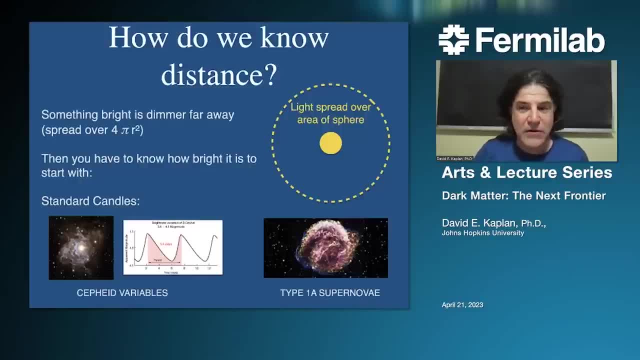 Which are objects whose Whose light or amount of intensity that is emitted corresponds to some other property of it. So in the case of Cepheid variables, these are stars whose brightness fluctuates, And there seems to be a direct relationship between the fluctuation of the brightness and the average intensity of these things. 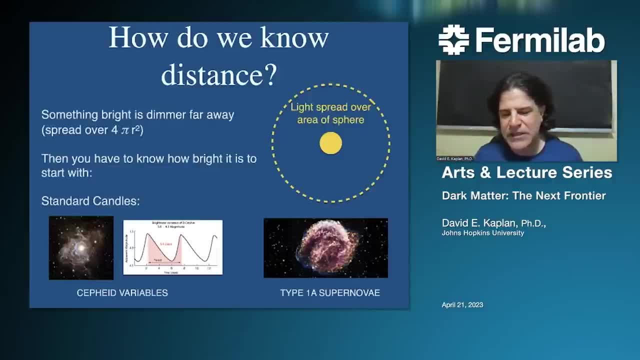 Another thing that seems to be a standard candle or type 1a supernovae. A supernovae Supernovae is a star that explodes, And type 1a is a special kind. It's a white dwarf, which is a dead star around the mass of the sun. 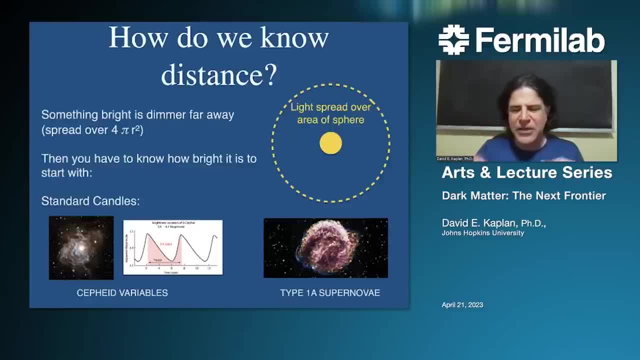 Which, if it collects enough matter, say from a neighboring star, it gets above a certain threshold, Which is about 1.39 times the mass of our sun. And as soon as it gets above that threshold it begins the process of nuclear burning and then exploding. 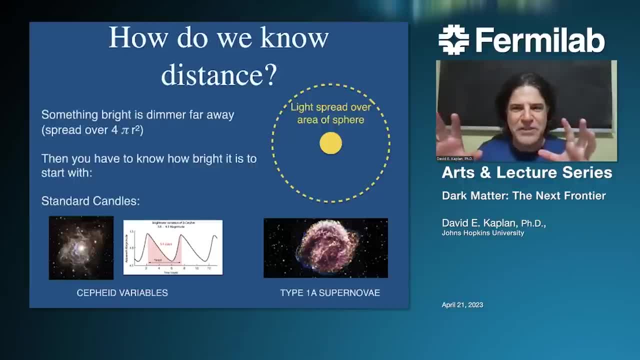 And because That number is quite precise, the idea is that these explosions happen with always the same amount of energy. There are some fudge factors in these things and these are complicated systems, But it has allowed us to map out to very far distances using very bright objects. 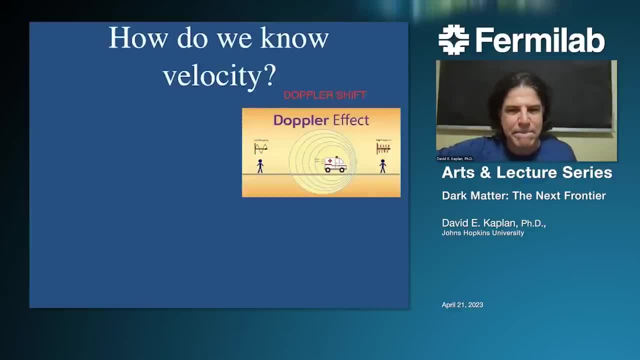 Most importantly, an exploding star in a distant galaxy. Then you can ask: how do we know velocity? How do we know how fast something is moving away from us? And this is actually easier than you might expect. There is something called the Doppler shift, which you probably have heard of. 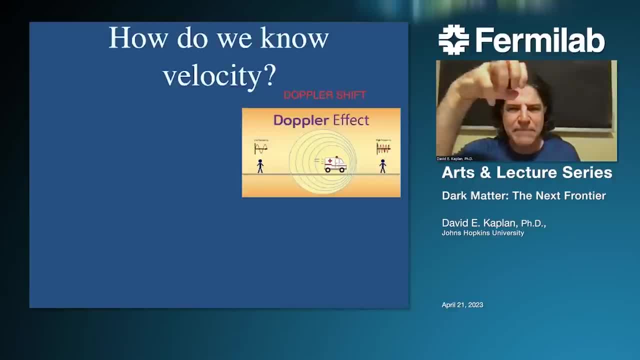 Which is the fact that if a wave is being emitted by something which is, say, moving towards you, Then the wave that's coming towards you is squeezed And the- let's say- peaks of the wave are arriving faster than they would have if the source was standing still. 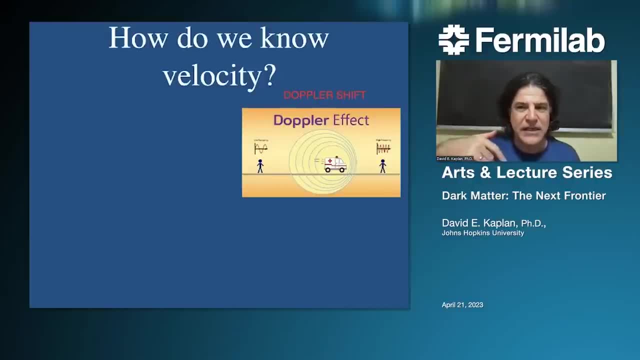 So it looks like the frequency of these waves is increased. Or, if you're behind it, if it's moving away from you, they're stretched out And the frequency of those waves are decreased. So if you have a source that emits a wave at a certain frequency and the source is moving away, 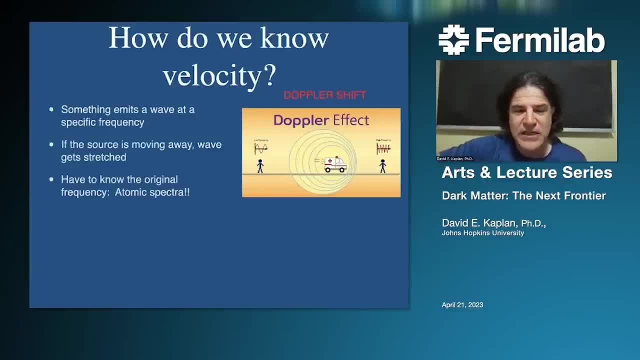 that frequency will appear to be less than what you expect. And now we can ask: are there frequencies that we know for sure? And the answer is yes. atomic spectra. Light gets emitted from gases of atoms, And atoms, because of their quantum nature, have very specific energy transitions. 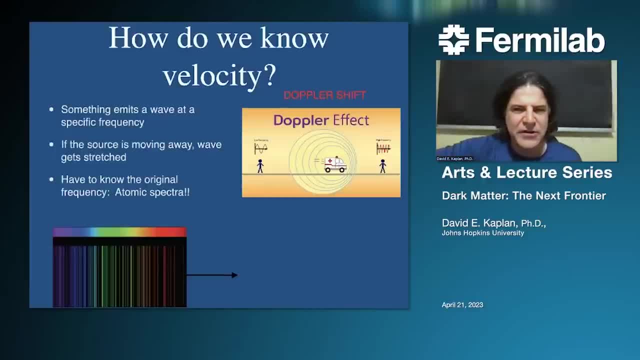 All hydrogen atoms have exactly the same different energy transitions And those transitions emit light, And the light is of a specific frequency which is proportional to the energy. And therefore, when you look at a gas of hydrogen or any specific type of atom, 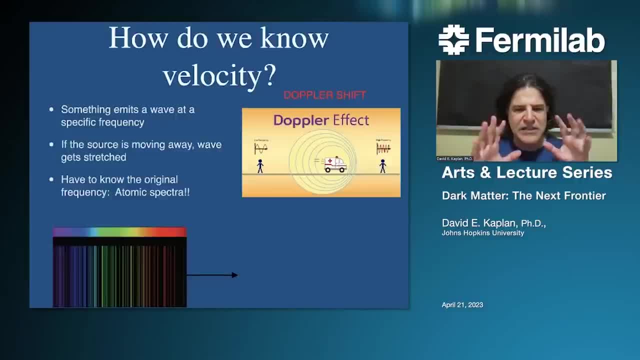 you see a well-defined set of lines spaced in a very specific way. It's sort of like a barcode when you're buying something in a scanner So you can immediately tell what type of gas it is. But if you see all of those lines in the perfect pattern, but they're all shifted. 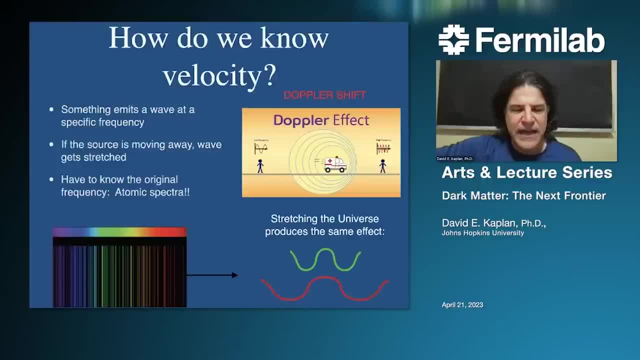 to a different wavelength or a different frequency, then you know you're seeing hydrogen, but the light that's coming from it is emitted by something that's moving either away from you or towards you. We call that redshifting: It shifts towards you. 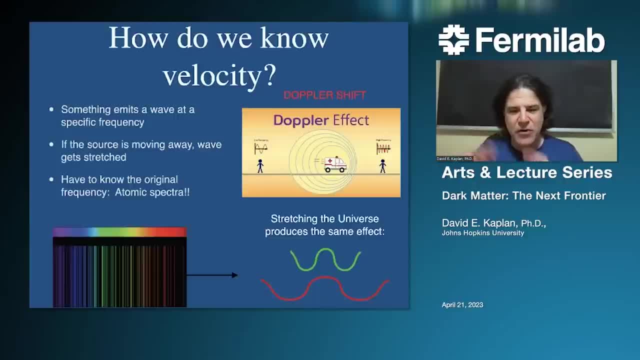 It shifts towards you, It shifts towards the red, which are lower frequency or longer wavelength. And this happens not only because of velocity- something moving- but if the universe is expanding it also stretches out these waves and produces lower frequency light. So you can tell how fast something is moving away from you or how much the universe has. 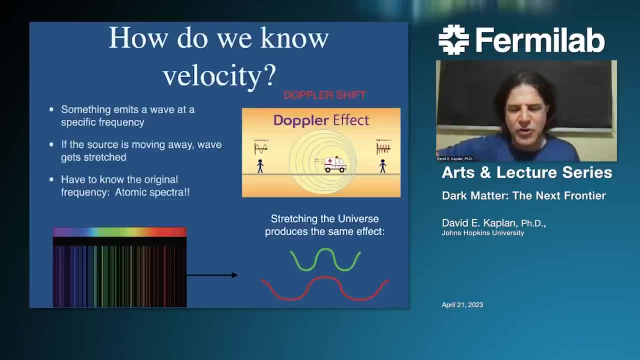 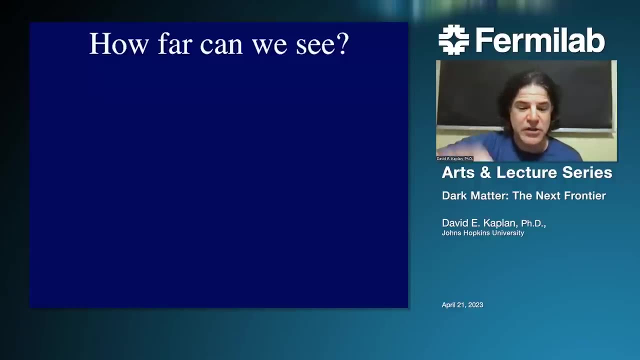 expanded between the time it was emitted and when you measure it, by how stretched these waves are, how much The frequency bands have shifted towards the red colors. Now, how far can we see? We look into the universe. We see a whole bunch of galaxies. 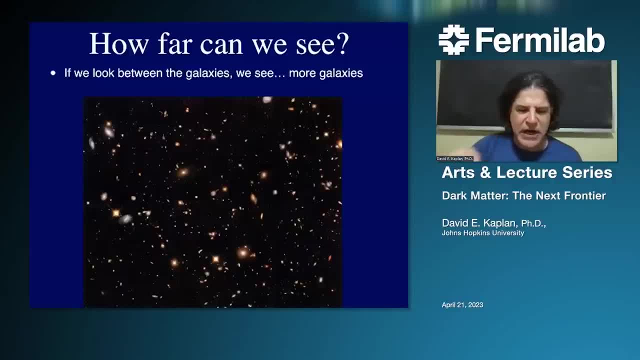 Famously. when the Hubble telescope started operation, it found the darkest patch in the sky and opened its lens for exposure for a long time to see what it could see, And it saw something like this: Loads of galaxies That if you look farther and farther you can still see them. 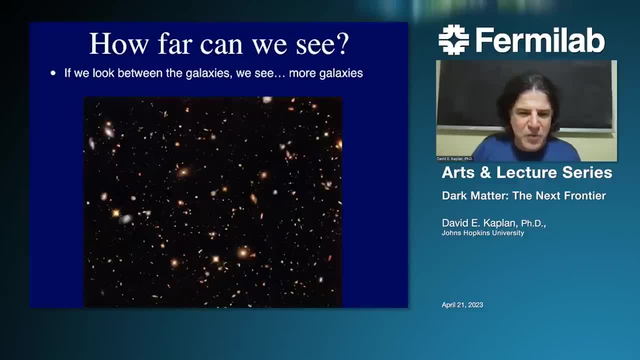 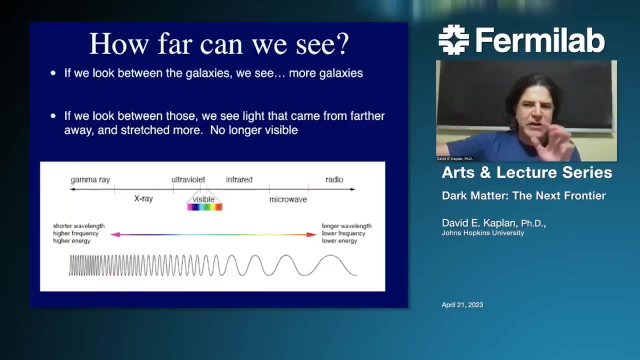 They're dimmer, but they're there. And so then you can ask: well, what if I look in between the galaxies, Could I see anything else? And because the farther out you look, either you could describe it as the moving faster away from you or, better yet, the universe had more time to stretch. 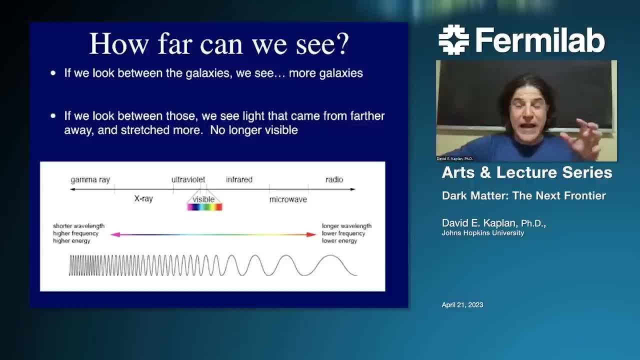 Eventually the frequency of that light is no longer red, It goes to the infrared. It can keep moving, It can keep stretching into very low frequency light or very long wavelength that we can't see and see with telescopes, but we can in principle detect it. 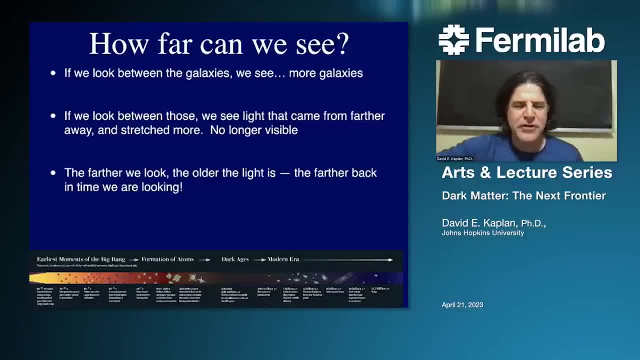 Now, if you look farther and farther, you're looking at light that got emitted longer and longer time ago, because light travels at a finite speed and therefore you're seeing older and older light. That means you're seeing light emitted in an earlier and earlier time. 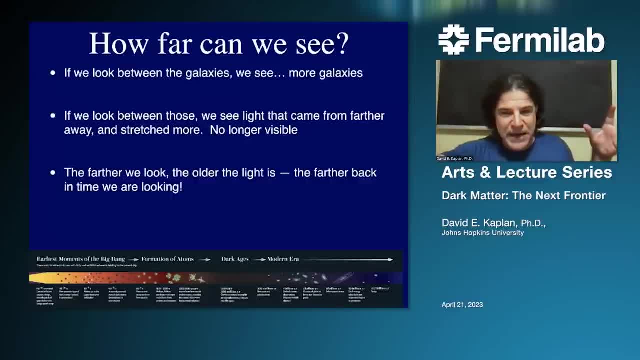 In the universe and if the universe was expanding for a long time. very early times the universe was actually quite dense And in fact You could look all the way back to a time when the universe was so dense in between all those galaxies. 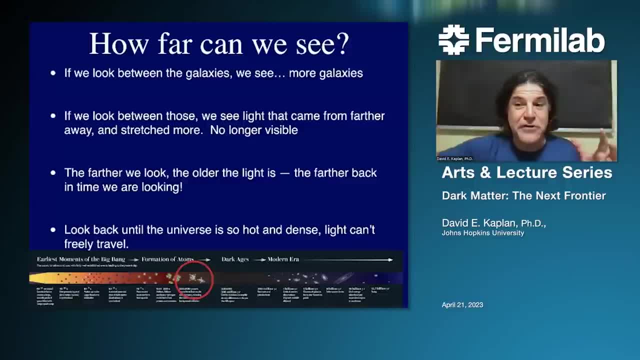 That it The light itself can't traverse the universe. You can look back to a time when the temperature of the universe The same as the temperature of the surface of our sun. So there is a time back then when the entire universe was basically one big star and light doesn't travel in straight lines inside of stars, it bounces around until it gets emitted from the surface. 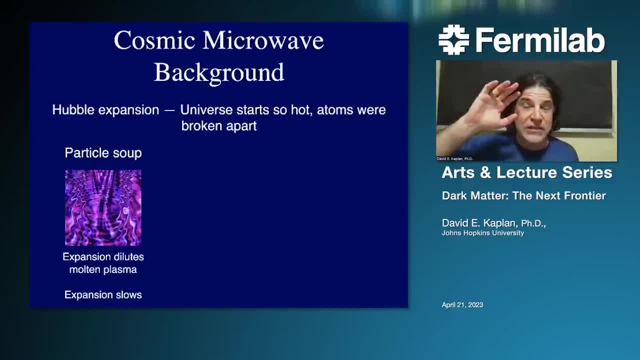 And so what you imagine is in the very early universe there is some soup of the matter, the atoms and the particles and the light, and as it expands it cools and things calm down and coalesce and light can travel. And the moment that light can start traveling is the moment after atoms can form. 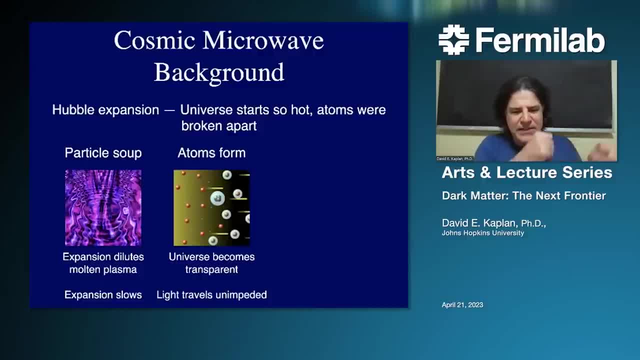 So when the universe is super hot, it means everything. Everything is crashing into each other at such high energies that it is breaking apart atoms and atoms can't form into their stable states. And when you have a bunch of charged particles around, a plasma light bounces all over the place. 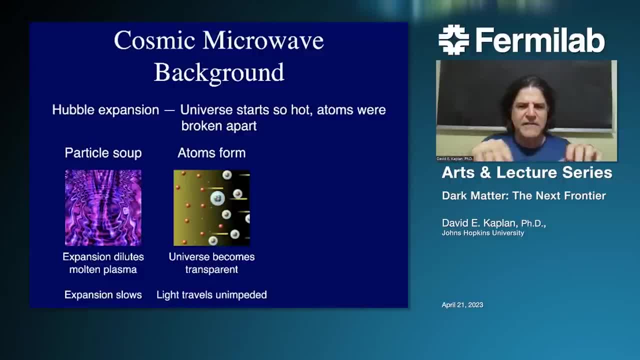 But when the atoms form and the energy in the light is low enough that they can't excite the atoms, they just travel through them as if they are transparent. Light has to be energetic enough to be able to excite atoms, The way visible light can excite molecules and atoms in our eyes. 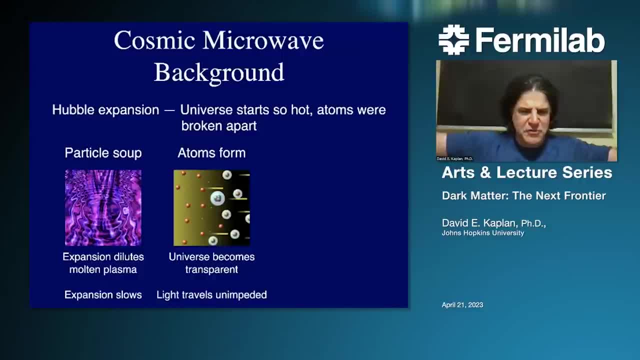 And therefore there will be a time in the universe where the universe was cold enough that light just passes through. the universe becomes transparent, And that's at a specific time, which means if you look back far enough, you will see a surface. 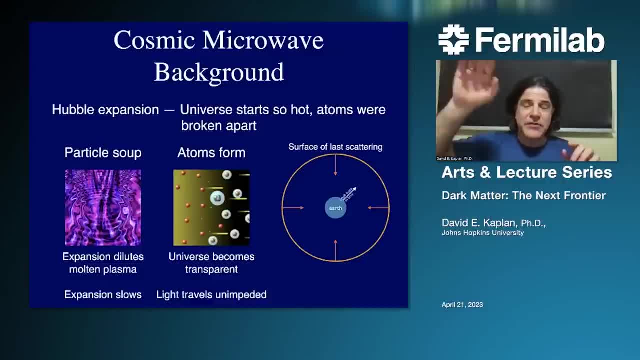 We call that the surface of last scattering, That is, back when the universe was like a giant star And now you're seeing that When the light last was bouncing off of all the components of the universe and now can just travel straight in random directions. 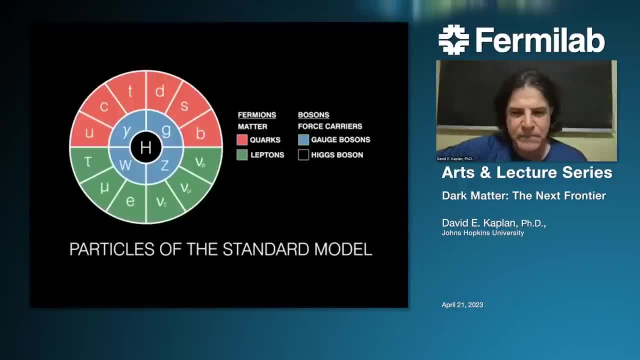 And we? for us it looks like a surface, All right. So that's how we do astrophysics, cosmology, in the sense of how we see things and what we see out there. And now the other thing we need to know is basically the laws of nature. 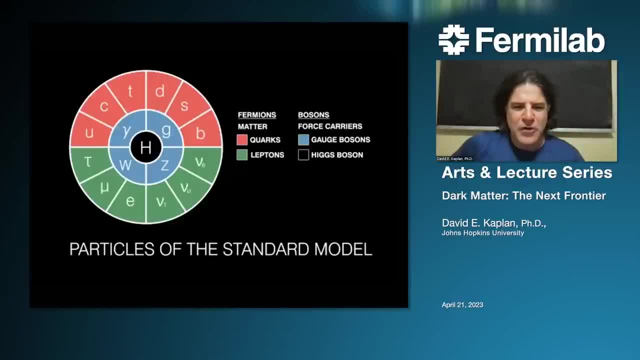 And I'll just give a one slide picture of that, Which is that there is a lithograph, There's a list of particles which we call the standard model. A standard model is that list which are quarks and leptons and force carriers and the Higgs boson and their interactions, how strongly they interact with each other, plus the underbelly, which is quantum field theory. 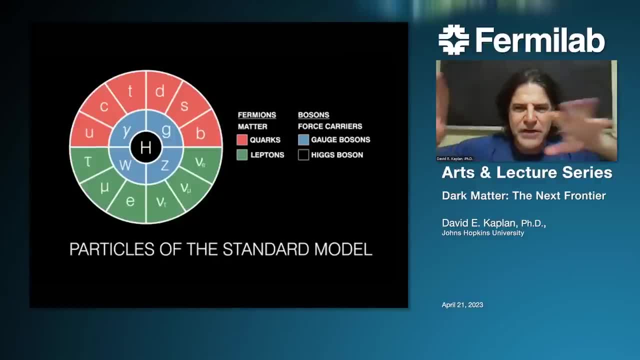 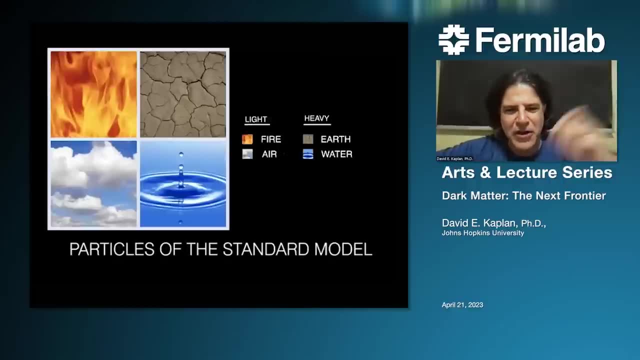 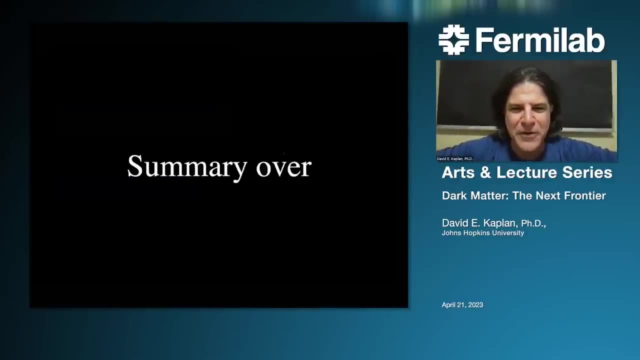 That's the known fundamental laws, And so, whatever those are, they should describe how matter works in the universe, And this, you could say, Replace the old set of laws, which looked much simpler, but the math turns out to be much more complicated if you describe it in the old way. that's the summary. that's just a summary of the basic pieces that we know. 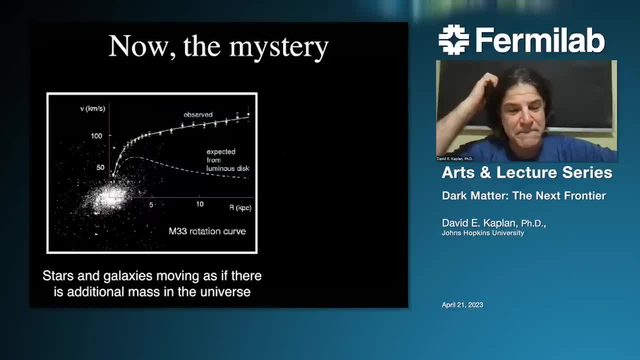 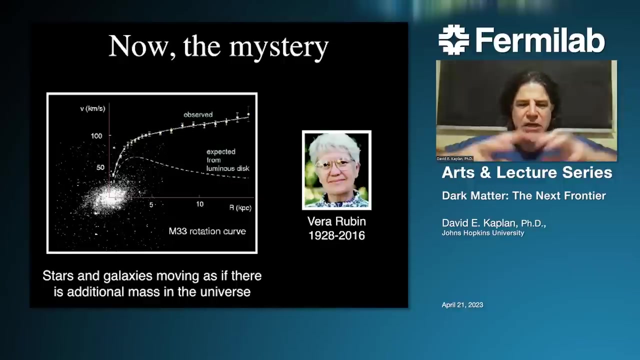 And now the mystery. So there's a mystery Which was discovered long ago by a few people. The probably the most accurate analysis Statistically in the early days was by Vera Rubin in the seventies. She was measuring velocity curves. What I mean by that is you can look at a galaxy and you can ask what is the velocity of various stars towards the center of a spiral galaxy, say, and then out to the edges. 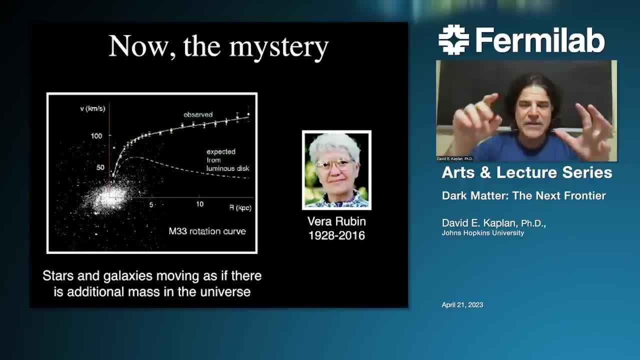 And in those measurements what you would have guessed happens is if something is far away from the center- Let's say you have a mass there- The earth is traveling around the sun. If you're farther away, to travel in a circular orbit, you're going much slower, because if you're going too fast but the force is very weak, you go flying off. 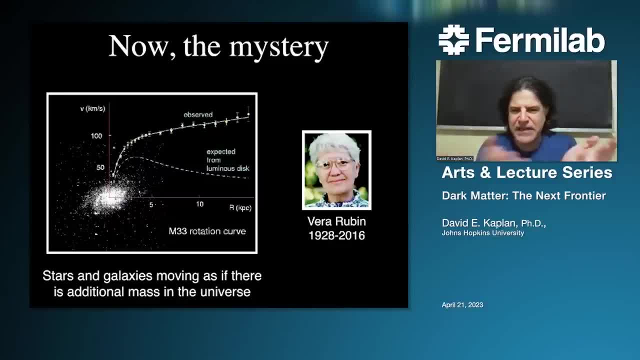 So that's why, for example, the earth's years, 365 days, mercury, which is much closer to about 80 something, And then the far planets out there is like 10 years, something like that. So that just has to do with the weaker force: the slower you can go and still be in orbit. 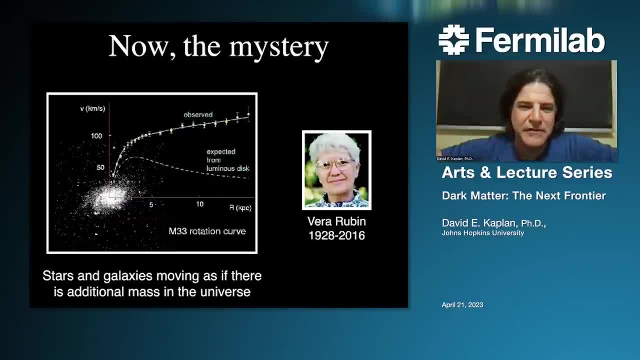 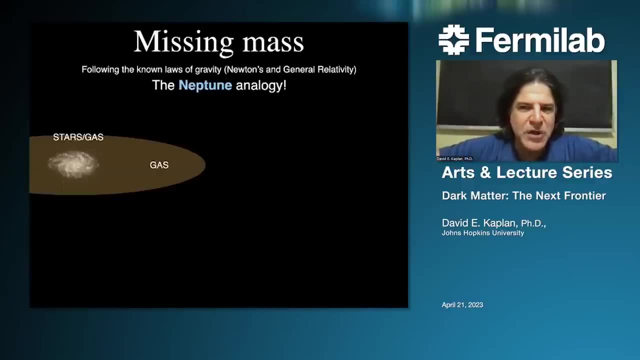 And instead She was finding roughly flat velocity curves that you go farther and farther out, far away from all the visible stuff, and you're still going the same velocity. So it doesn't make sense. Something was wrong here in this description, And so then we can sort of make the historical analogy and say: well, what did Laverie see? 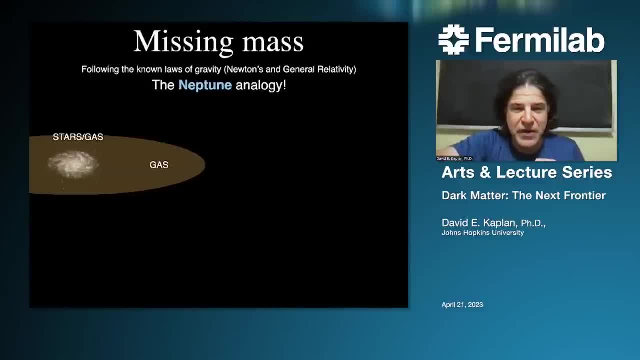 He saw something wrong with the orbits of, in this case, Uranus. And so if we make that analogy, we can ask: well, I know the laws of gravity, Newton's laws and general relativity. I know that the stuff is there, but there must be some other stuff in order to explain the paths, the orbits that the, both the stars, take, but also the gas which we can see and emits light and goes way out to far reaches of these spiral galaxies. 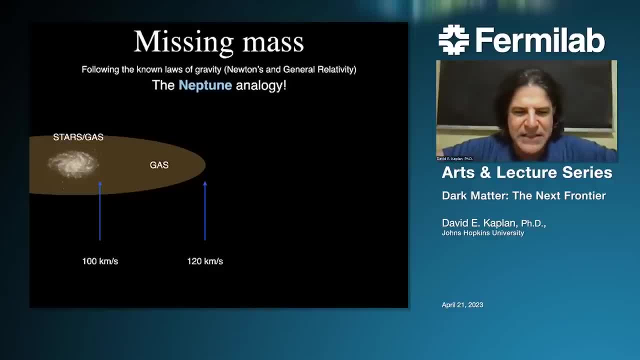 And we find that the light. so this is that particular galaxy coming from the far away. Gas is moving at the same, The same velocity, or even a little faster, but is bound to the galaxy, And that suggests in analogy that there's some other matter there. 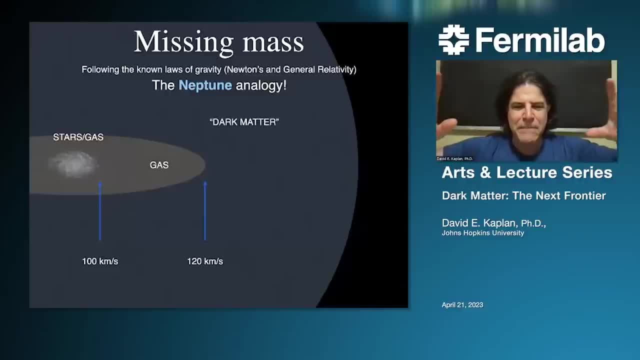 We're going to just call it dark matter because we don't see it. but lots more matter would explain these orbits. It's sort of the dumbest thing you could think. thing is going too fast. There must be more mass. We can't see it. 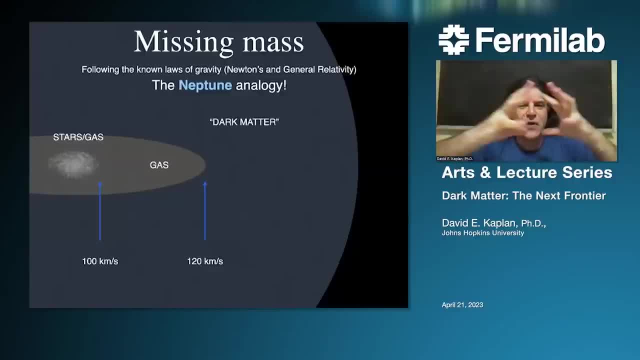 Let's just pretend there's more mass and it's distributed in a funny way. It's distributed all the way out, way beyond the stuff that we can see, And its density is not falling off too fast, And not particular for galaxies but for clusters. Fritz Zwicky is the first to to coin this. 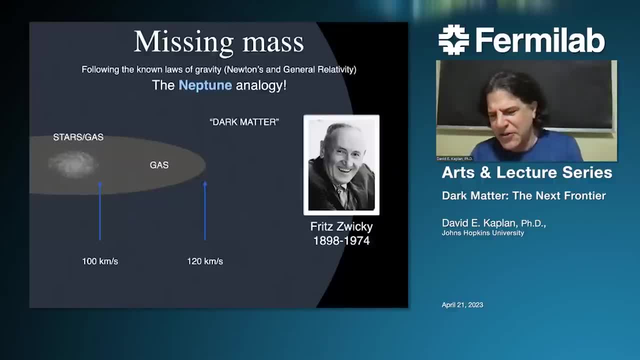 Although probably did it in German- He's a Swiss physicist- in the thirties noticed- I think it was the coma cluster- galaxies Weren't moving in a way to be explained by the local matter. Those measurements were not good enough to really say something concrete. 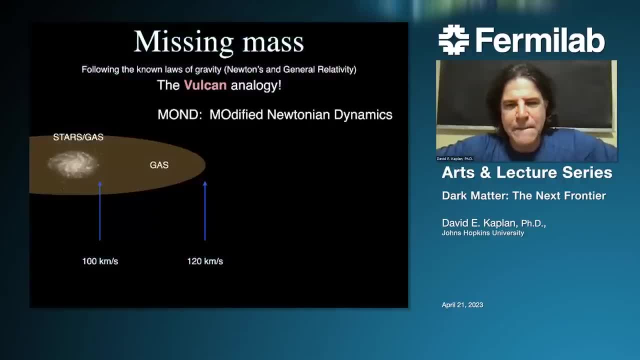 But the measurements in the 70s were. Now you could decide. well, maybe it's the wrong analogy, Maybe it's the Vulcan analogy. We see some different motion. We use the standard laws of gravity and the standard laws of motion, but it has been proposed Another possibility is just. 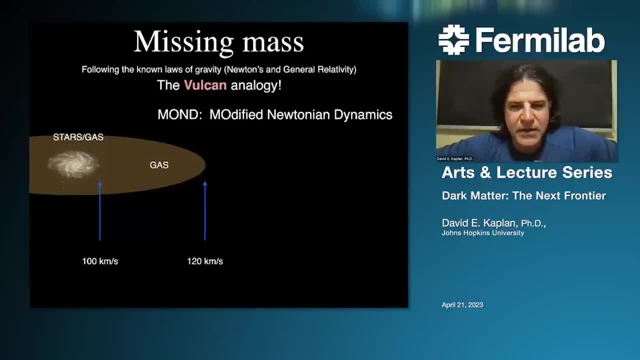 the laws of motion are just wrong, And a big proponent of this was Mordecai Milgram. um, who's still alive. He's at the Weizmann Institute. Um and uh, Mordecai was suggesting that these laws for very low accelerations are different than the famous. 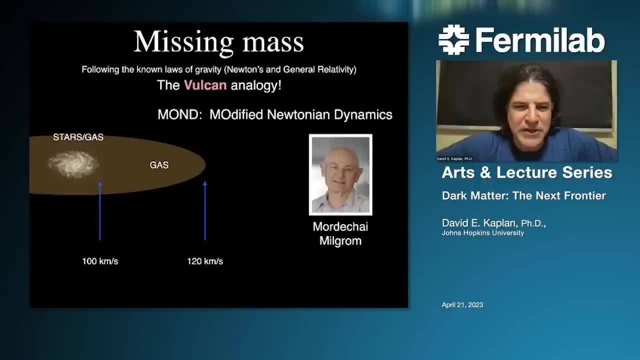 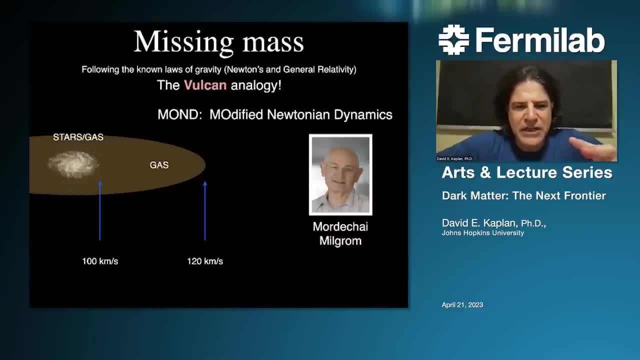 the distribution of the dark matter that you would need in each one kind of looks a little bit accidental that you get these flat velocity curves for different size, both galaxies and clusters. So the Mond thing was something which, uh, you know you're doing something dramatic. 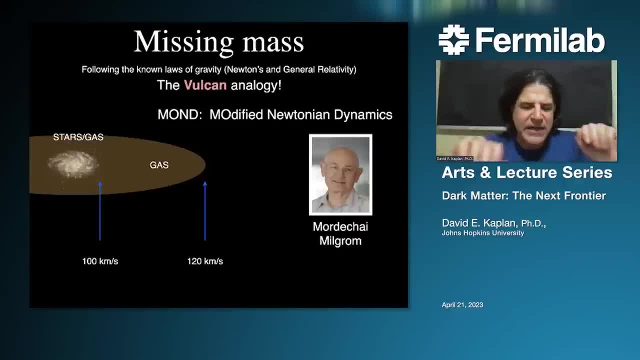 changing the laws. um, but it explains some nice uh data. Um. what was not easy for Mond was to incorporate it into general relativity. There was no clean theory that allowed that to happen, but people worked on it for many years. 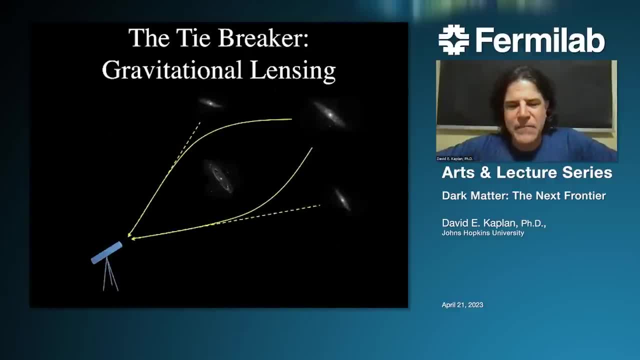 But then there was a tiebreaker, which is that uh, matter does other things too, And for one thing it, it lenses light. So this is a general relativistic effect. And the general relativistic effect is that if you look at an object far away and there's some massive object nearby, 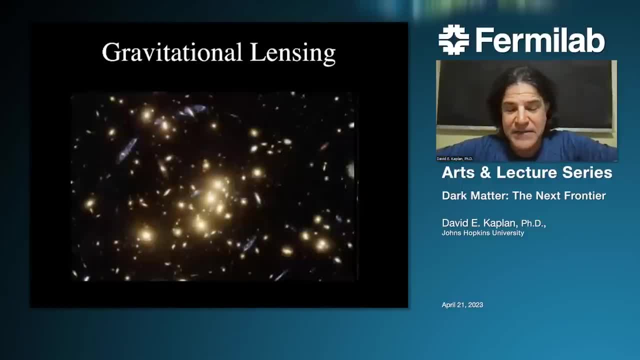 the light will bend And you can see, in fact, very dramatic cases of this. You have a cluster of galaxies. Um, here's a lens with a cluster in the front and then the blue blobs there is from a galaxy behind it being lensed, And so the lens is not only works the galaxy, but it makes multiple. 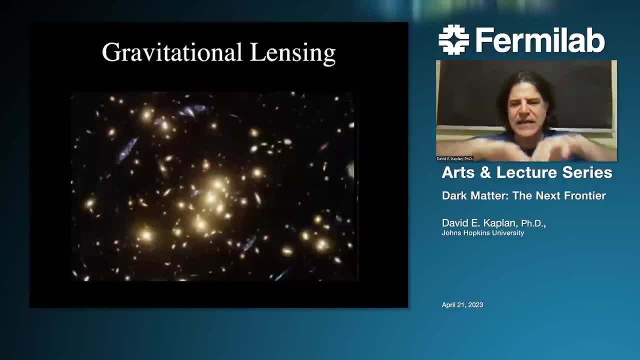 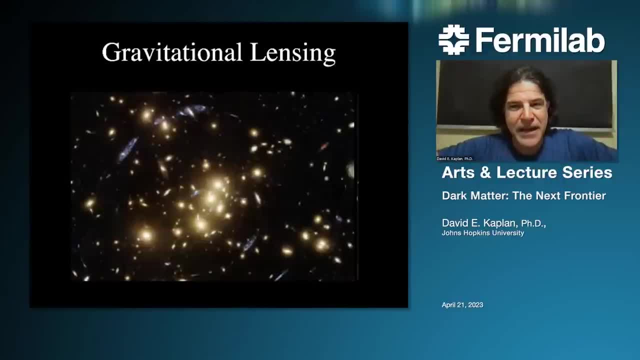 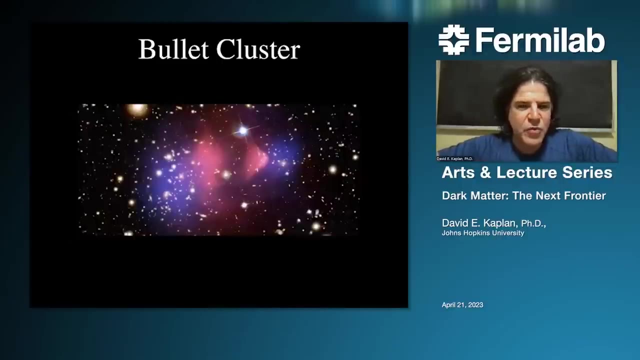 of weighing the mass of a cluster And we see masses which are much larger than the mass of the stars and the even more important gas that lives in these galaxies. A very dramatic effect like this is something called the bullet cluster, which were really two clusters that have been 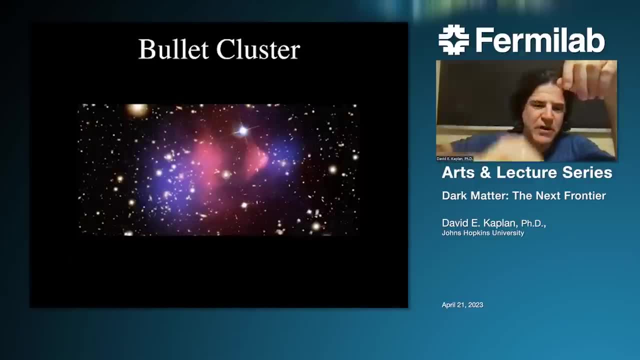 seen a smaller one which plowed through a larger one And that weird sort of triangular shape of that uh pink blob Is due to the friction of the gas of the smaller cluster plowing through the bigger one And because of the friction it's slowed down And the majority of the mass of the visible matter. 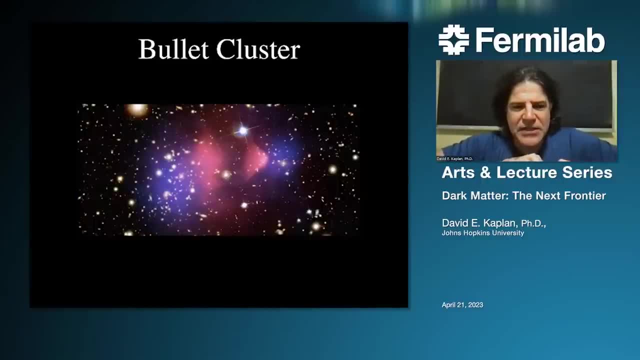 turns out to be in the gas, um, and not in the stars, which can really flow and don't hit each other. It's so dilute but most of the mass was in that gas and the gas slowed down, but the stars 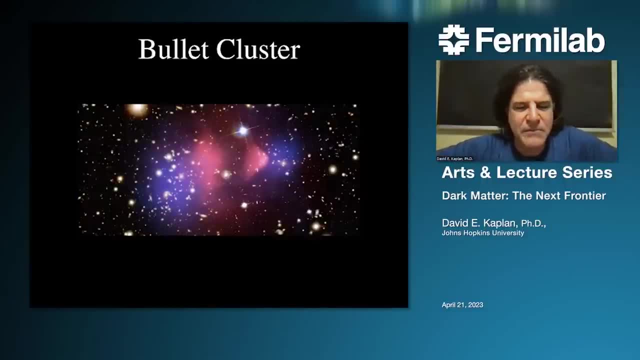 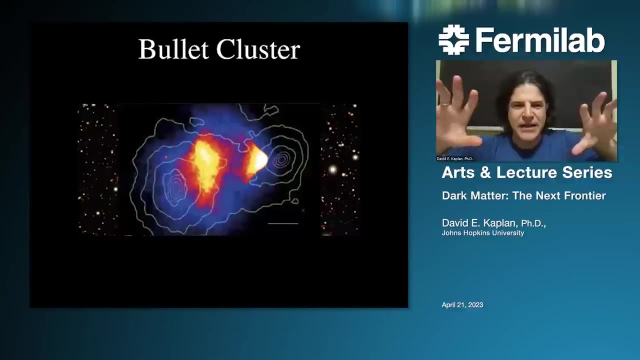 could keep going. But now you can take the bullet cluster and you do a lens. What makes the bullet cluster so fantastic is that it actually is lensing some visible galaxy behind it And when you map out where the mass is, uh, due to the lens, the mass has plowed through and you see on the left and 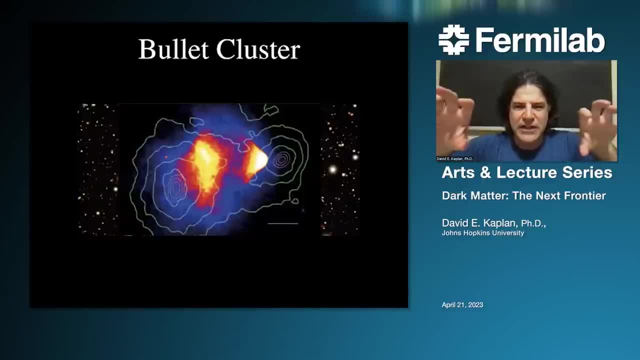 right the centers of the mass of the two clusters, and they're not where the centers of the mass of the gas is. So the gas slowed down due to the friction, but some other kind of matter just passed through without friction and kept going, And so this is even more striking evidence that there's stuff. 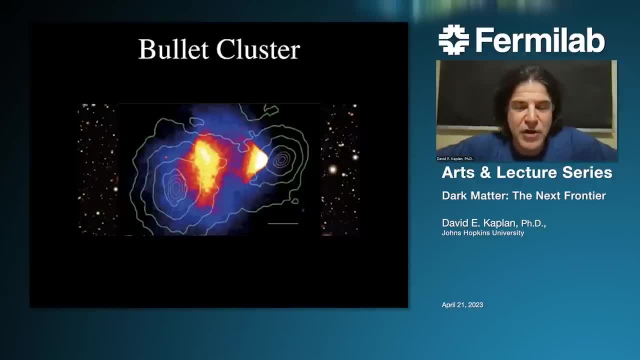 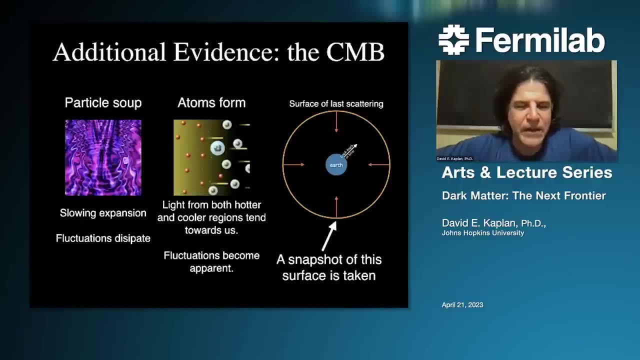 there that doesn't interact with light and and doesn't strongly interact even with itself, Um, depending on its mass. but an even more uh compelling piece or dramatic piece of evidence For the existence of some kind of dark matter is the light that comes from the surface of. 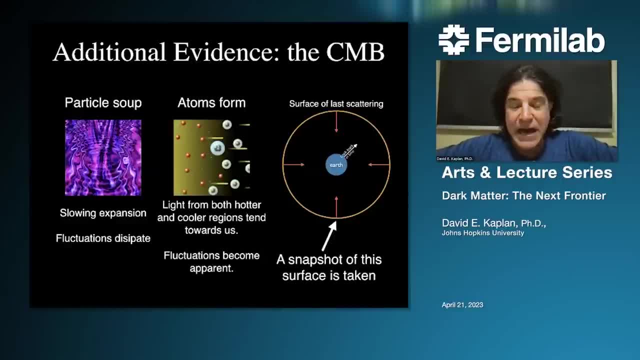 last scattering, which we call the cosmic microwave background because it's in microwave frequencies. The point is that when the plasma was expanding and sort of fluctuating, it's this plasma, So there are waves in it as it expands and cools And eventually, um, it cools so much. 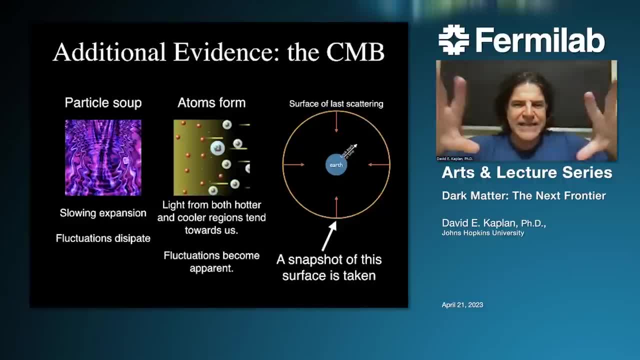 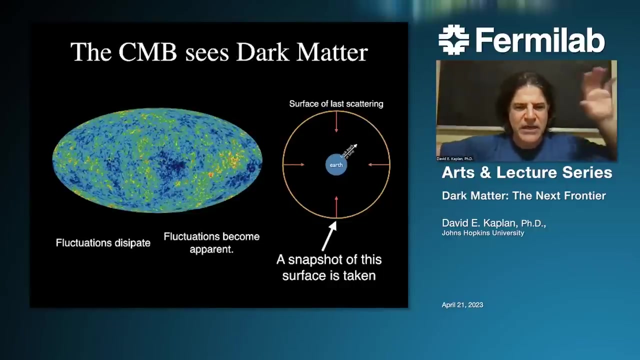 that light gets released from it. That light It gets released imprints the information locally of what the temperature was. And if there were waves in that soup then the temperature from different parts of that surface is slightly different And we've been able to make maps of the entire microwave background. And if you 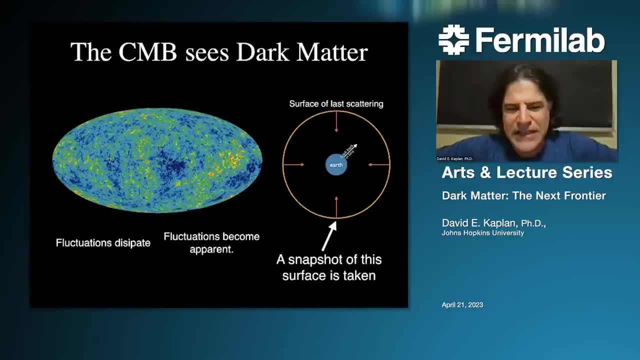 subtract out or average out the temperature. uh, let's say the green color is roughly the same as the average temperature. Then the from the dark blue to the red are fluctuations of about 10 parts in a million. So the temperature is almost perfectly uniform, but there are tiny fluctuations and you can see kind of how it's speckled, that there's sort of a favorite distance between dots. The shortest distance, um, uh, dramatic typical distance between dots is roughly one degree on the sky. 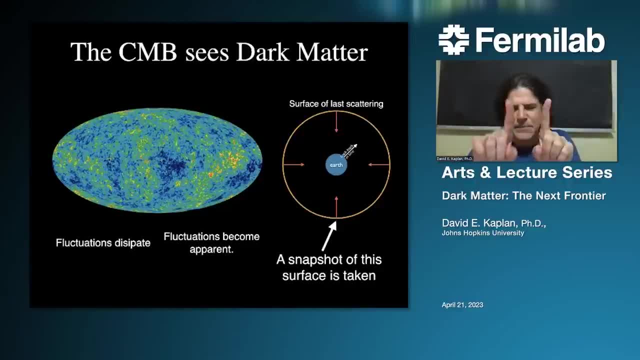 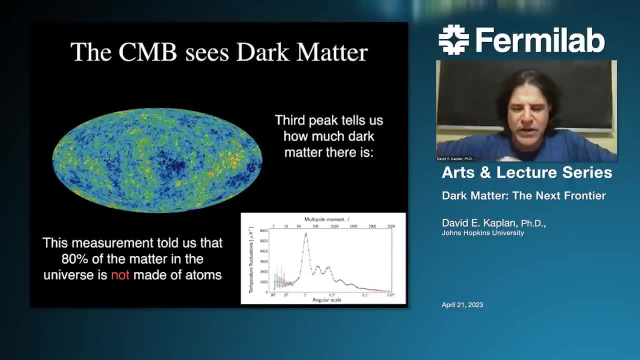 And so if you plot The sort of temperature times, temperature of different spots, different distances away from each other, you can map out in a mathematical plot Um, where the most typical distances between two points and those distances tell you what the um waves were doing at the time when the photons were released. 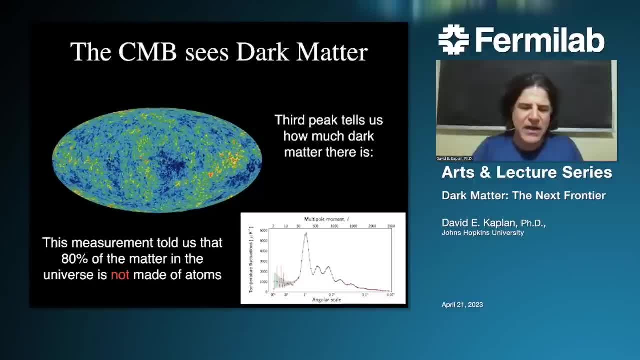 So what we see is a pattern, that that tells us a lot about what the dynamics of the fluid Or the plasma was at that time in the universe, Which contains information about what's in the universe. Uh, how fast the universe is expanding. 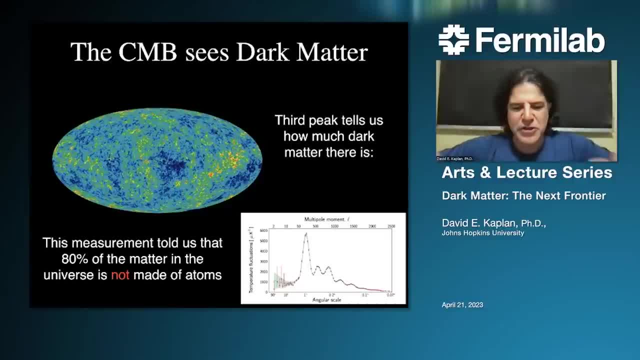 And the clumping of the universe which is caused by matter, but matter that feels no pressure, And so there is something in the universe, and this Uh careful study of the microwave background Gave us a rough idea of how much. 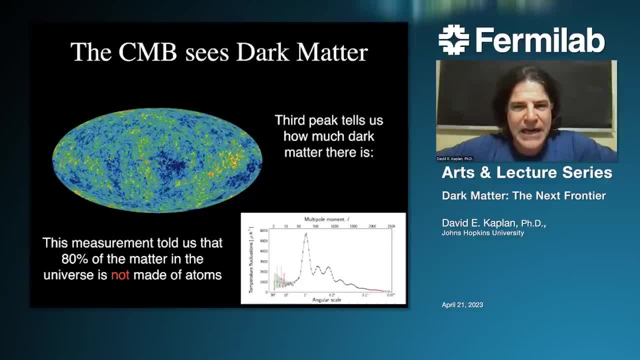 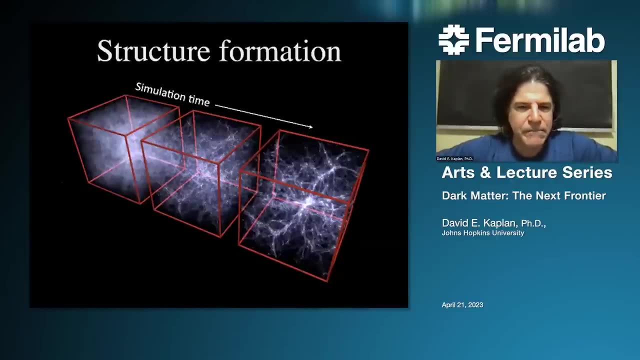 80% of the matter In the universe Cannot interact with light, Does not feel friction. Um, it must be made of something other than atoms, Because atoms Interact with light. We don't know what it is, And now you can simply take. 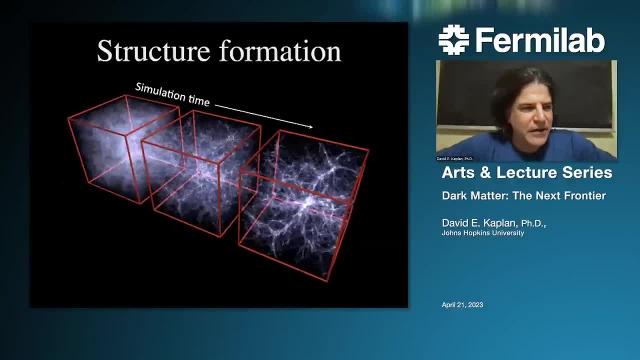 A, uh, mathematical, Uh model of this stuff. You just say, well, there's a bunch of stuff, It's in the universe. So I'm going to assume that it has little bits of fluctuations, Because it started with little fluctuations. 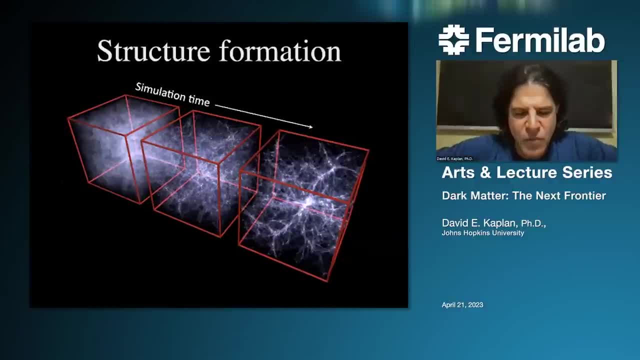 And, on a computer, simulate what it does. Uh, we discover, Um, that all kinds of structure gets created And in fact, the structure Uh looks a lot like. Uh, at its most dense points, Uh, what our universe looks like. 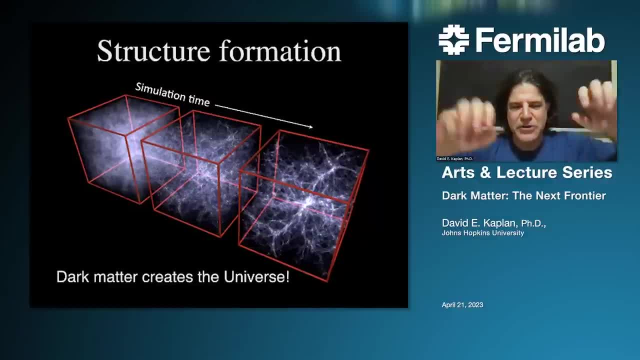 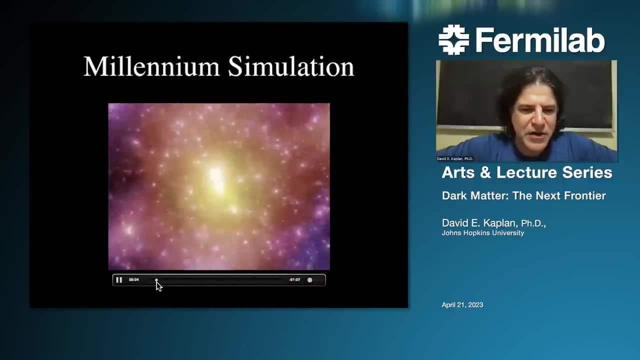 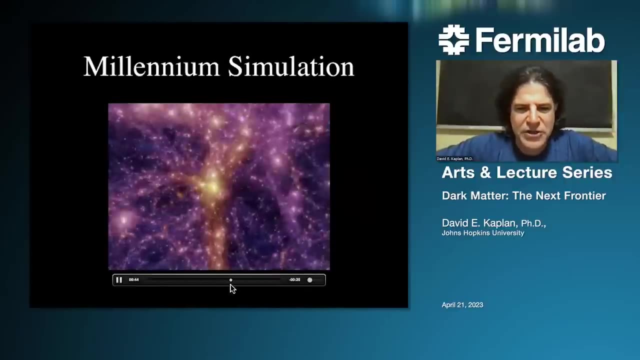 That structure being Clumps which produce, Um, both galaxies and clusters of galaxies. There's an old simulation- This is called the millennium simulation- And they simulated such a thing, And then that you could Create a three-dimensional Plot of this thing and see a video. 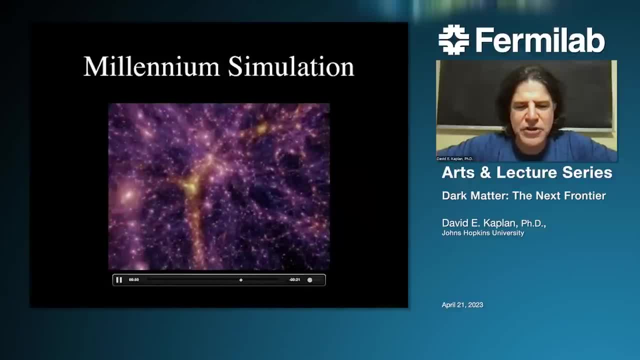 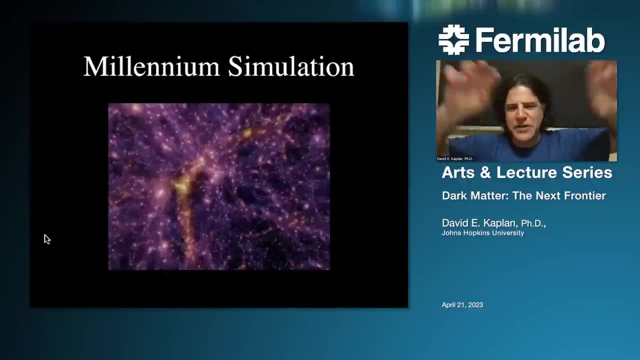 And what we've seen is not just that the distribution of galaxies Matches simulation like this, But even the filaments that go in between the densest regions Have now already been seen. Uh, using gravitational lensing, So we've already now. 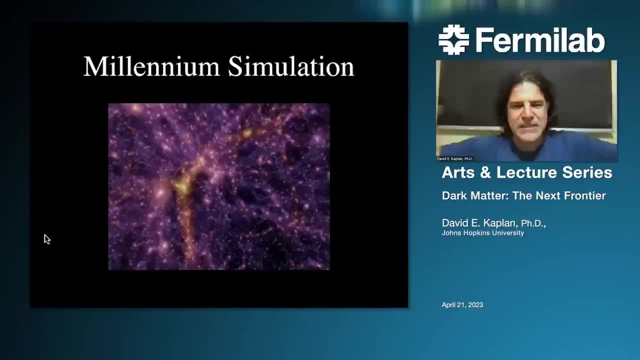 Uh, I'm not sure what we're seeing, But we're. We're going to see the structure of the dark matter, Whatever this matter is that lives underneath, Uh, the visible stuff, which is the stars, galaxies and the gas. 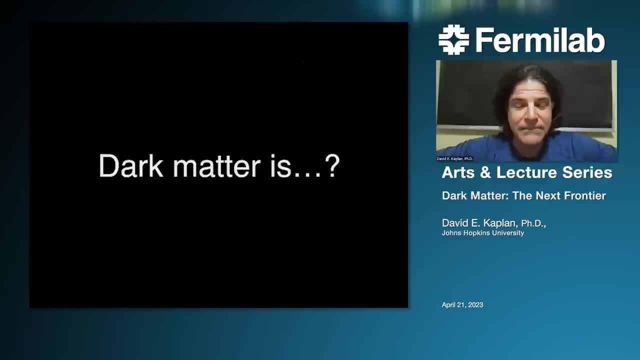 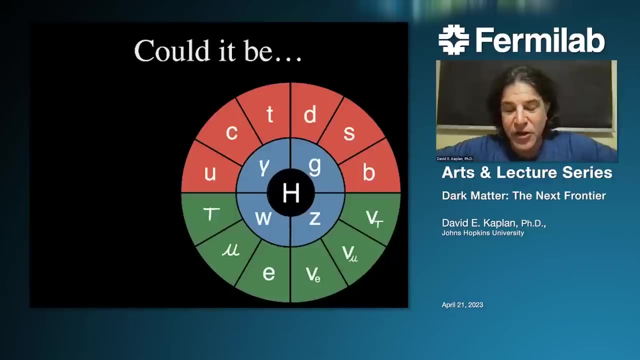 And dark batter is something else. We don't know what it is It's behind. feel responsible for it, because it's my job to figure out what the laws of nature are. Uh, my colleagues and other people in, and so this is what we're after. You could say: well, you know there's atoms, but there are all. 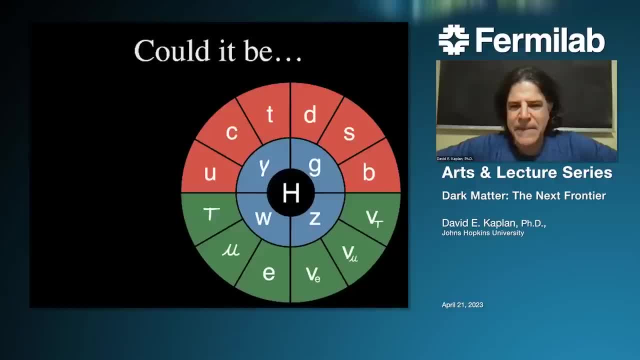 these particles that we discovered in giant colliders. and you could ask, are any of them nice candidates for dark matter? And most of these particles actually decay in a small fraction of a second, and so they would not be some relic left over from the early universe that's sitting around? 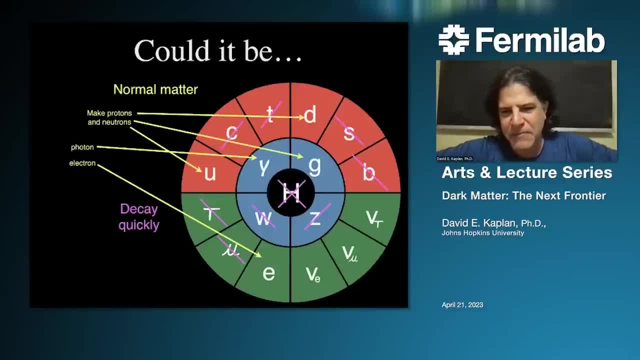 there today and living forever. Many of the remaining particles actually are normal matter. All the red particles are quarks and the U and D quarks. up and down quarks make up protons and neutrons, and the G, the gluon, is a particle that holds the protons and neutrons together. 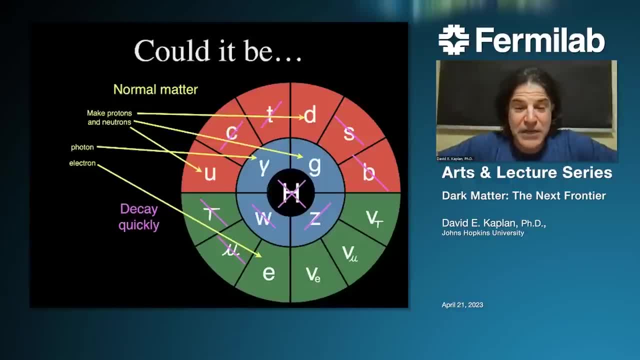 The electron, of course, is part of the atom and the photon is the particle of light. So all of these things which basically Make up the atoms can't be the dark matter by definition, because they're not dark. They interact dramatically with light or are light which leave something that potentially 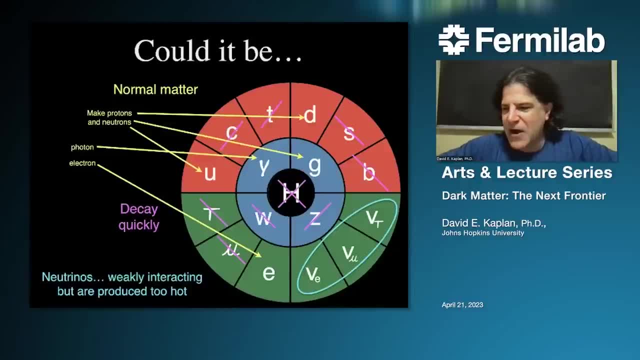 could have been the dark matter, which are the neutrinos. And now these neutrinos, which are very hard to see but emitted by the sun and should have been there in the early universe, unfortunately turn out to be too light And even though there's no way to know if they're, 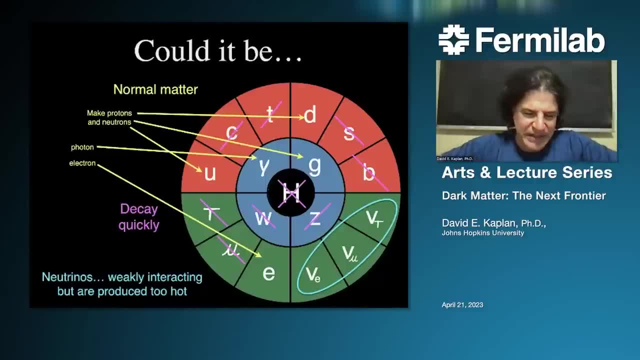 weakly interacting. they're still too strongly interacting with the standard model, in the sense that you can predict how hot and how fast-moving the neutrinos are today, and it's way too fast for these things to clump into galaxies. So that was our one shot. It's not that, It's something. 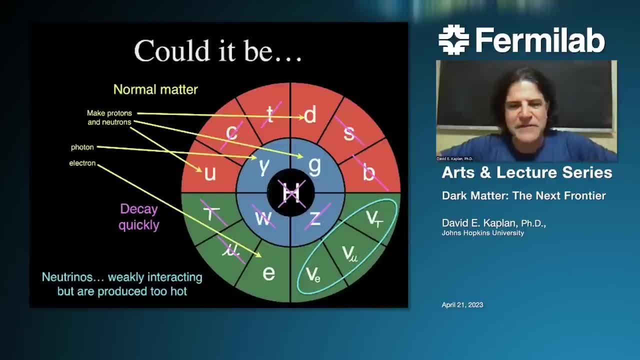 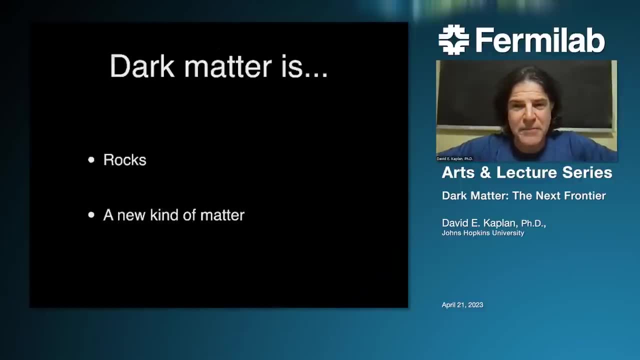 else. It's not made of anything in the list, It's not made of anything in the laws of nature, but we don't know what it is, So dark matter could be. I remember when I first explained this to members of my family, they say it's probably a bunch of rocks. You can't see rocks, you see. 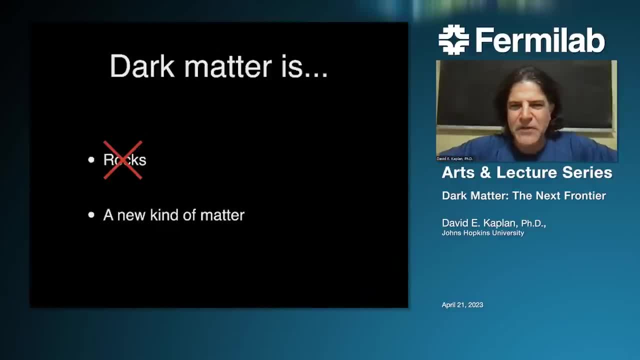 stars. so it's probably that. But that might have worked in the 70s, but now, because we know incredible detail about the expansion of the universe and a time when the universe was so hot- no matter what rock you give me, it would have. 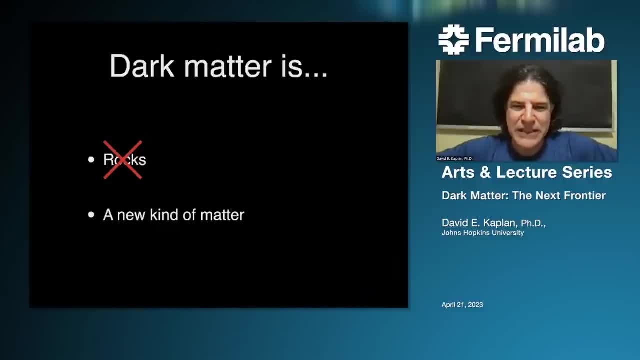 changed. So that's a good one. Melted and dissipated and vaporized in that early times, it's not rocks, Or if it's rocks, it's made not of atoms, it's made of something else, Or it's a gas of something else, It's. 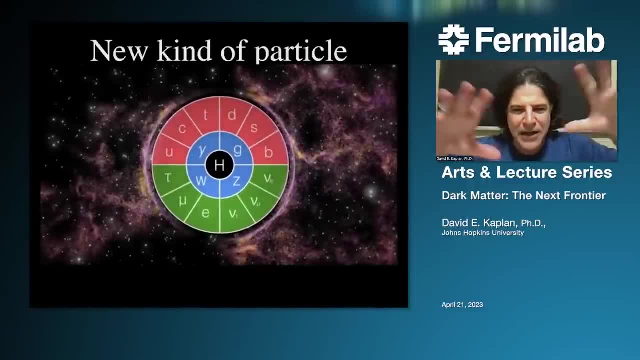 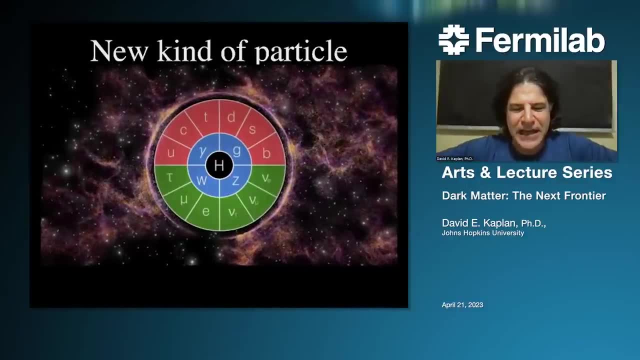 something new. It's some kind of new matter. So we would take our pretty little picture that we drew in a symmetric way that looks like that we've discovered everything, and then we have to add something else. So you could come up with some new type of particle and decide that new particle is. 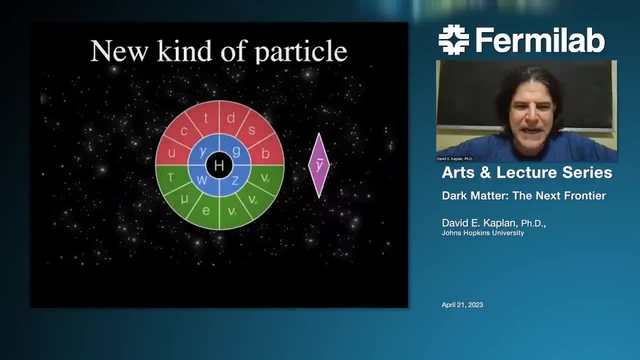 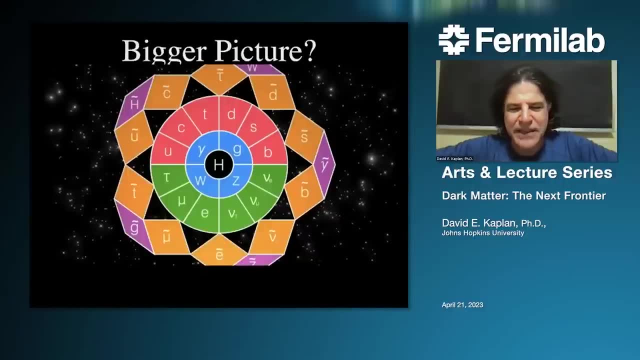 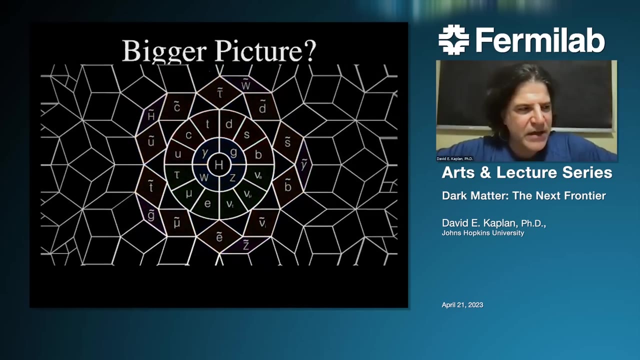 responsible for the dark matter and give it various fancy names, depending on your theory. And then, beyond that, people think about theories where a dark matter particle, some particle that could live forever, could be explained and explain even how much of the dark matter is. 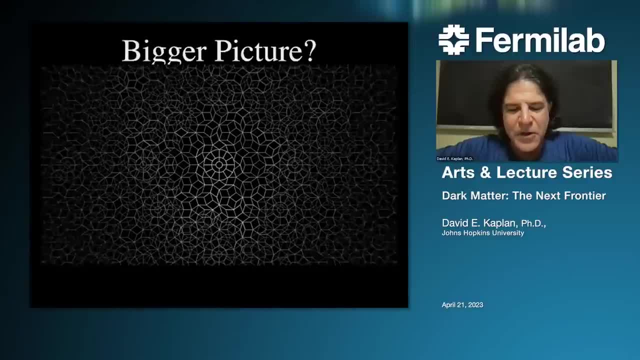 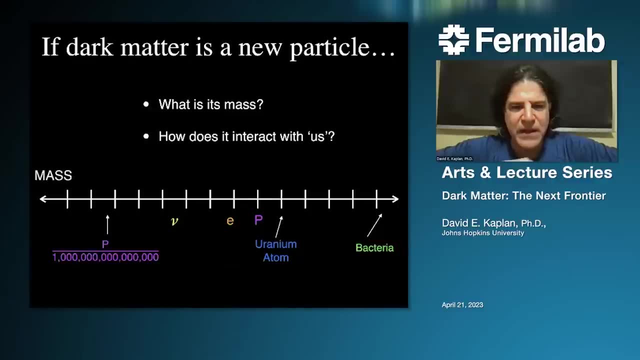 or various things you might want to try to explain. But really there's something new, something new in the laws of nature and something new in terms of the kind of matter, And the simplest thing to do is just to ask. well, 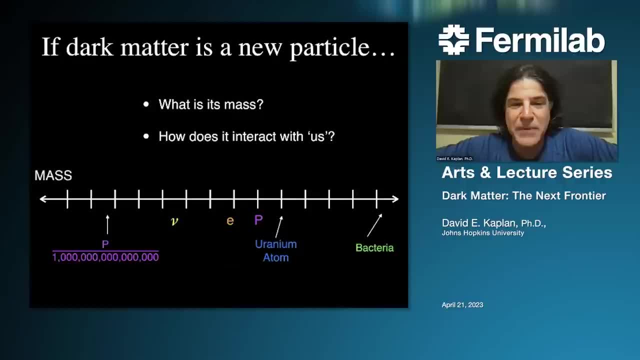 if there's a new type of particle that we just add to the standard model, we need to know what is its mass and does it interact with us in some way that is different than just through gravity? We've seen it gravitationally, but we'd like to know 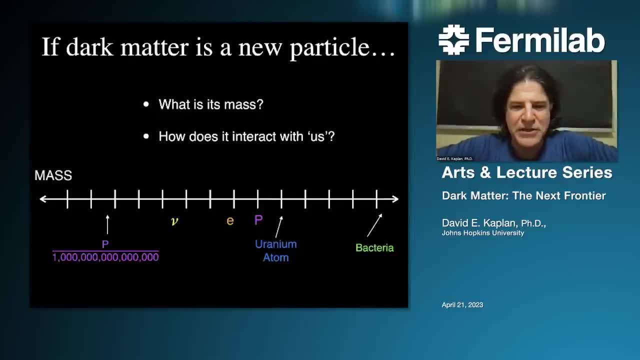 a little bit more about this particle and the information. How does it interact? How does it deeply live in the theory? Now our types of particles, particles that make up regular matter. there are protons, electrons, there's the neutrino down there And these 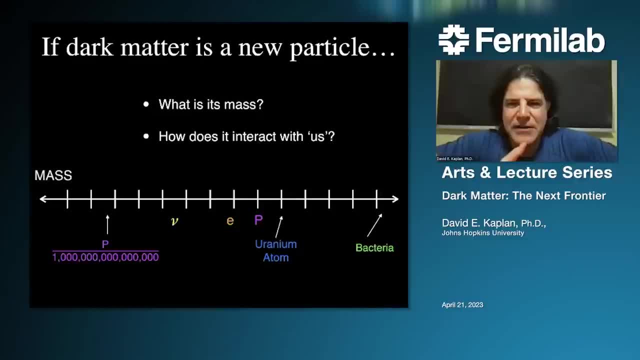 particles, you know, have a variety of masses. The electron's a thousand times lighter than the proton. The neutrino is more than a million times lighter than the electron. But if we're introducing a new particle, it could just be anything. It could be lots of different masses. 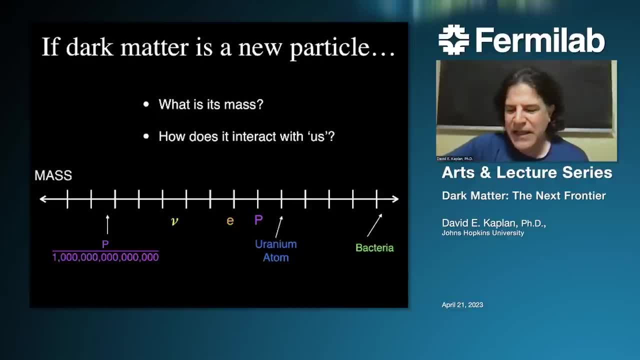 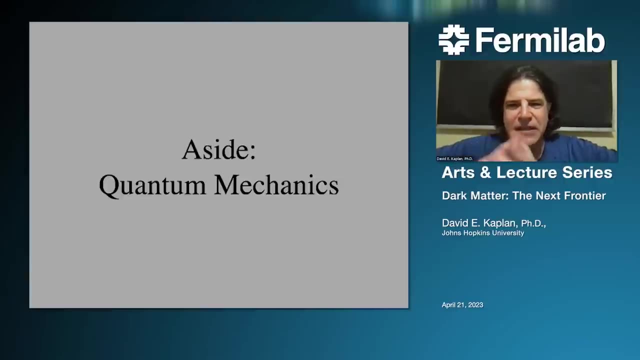 It could be trillions of times lighter than the proton. It could be heavy nucleus or even as heavy as a bacteria, or something like that. Now, if we're going to talk about particles that are extremely light, we need to have a little aside, And so let's just briefly introduce quantum mechanics. So 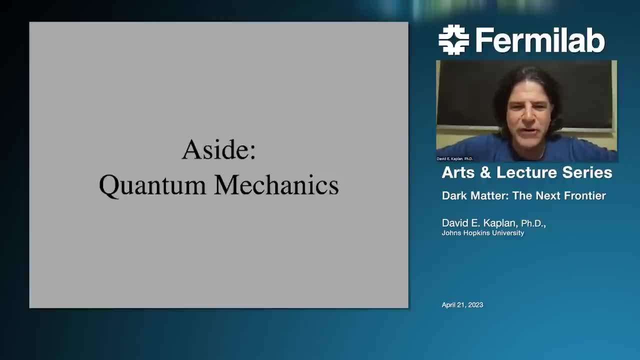 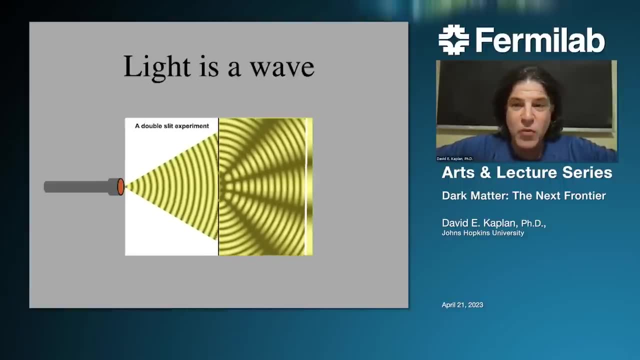 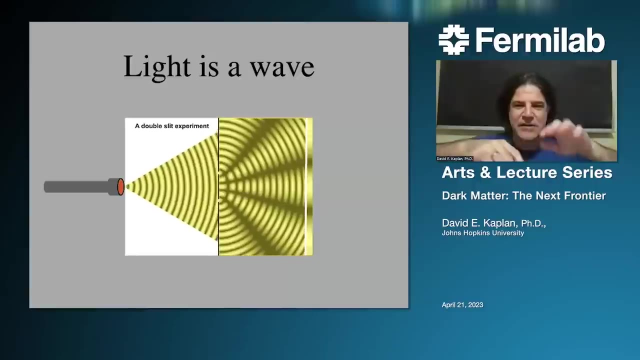 I'll teach you quantum mechanics in a couple of slides, and then we can move on. First thing you want to know is that light is a wave. What is a wave? It's something that has physical extent and it interferes. So light if the wave is set up just right. 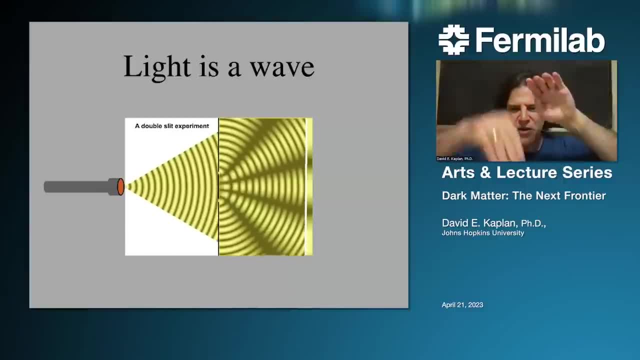 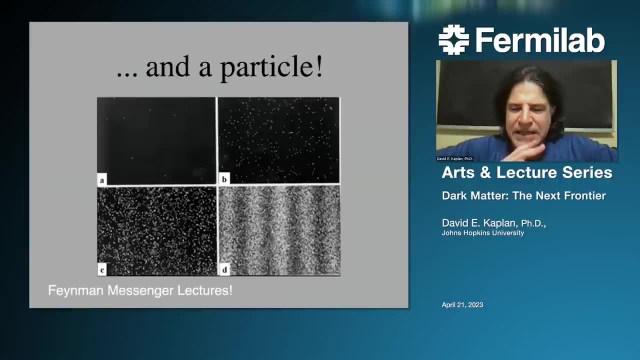 it can either constructively interfere, make bright spots, or destructively interfere and make dark spots on the screen, let's say to the far right. But the amazing thing is that light is also a particle And light is a particle evidence-wise. you can do the same experiment. 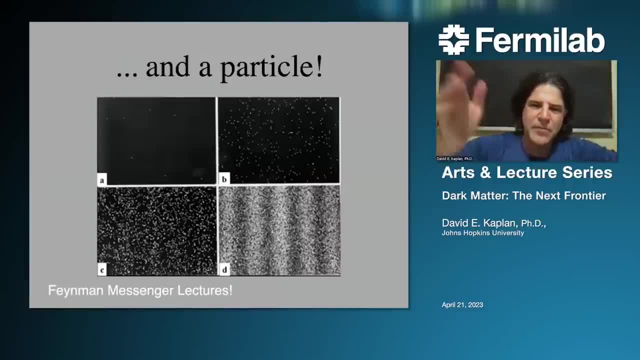 but turn the intensity of the light way down and put a photo detection screen there and leave the room and come back a week later or a month later And you slowly see individual bits, individual points building up on the screen, as if only. 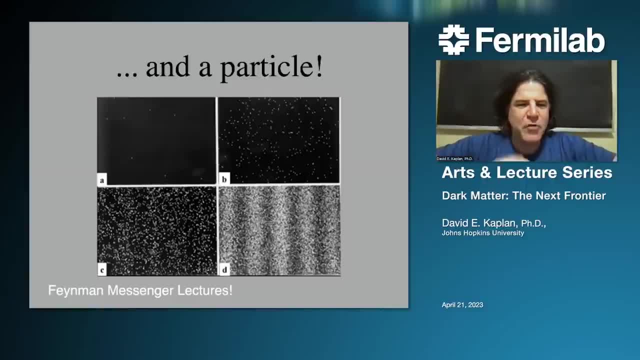 one particle of light comes at a time, And if you wait long enough, not only do you see a screen full of these bits, but you see the same interference pattern that you saw when the light was very bright, as if, even though, when it interacts with the screen, 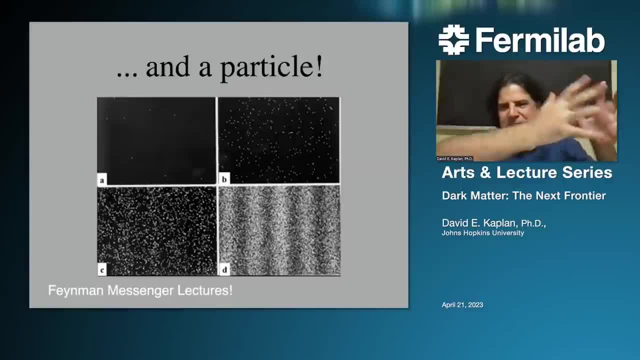 it's like a particle: it is behaving and it's an evolution from the source to the screen as a wave. This is a whole set of lectures and I recommend Feynman's Messenger lectures, which are free, and on YouTube or various sites, and they're beautiful. 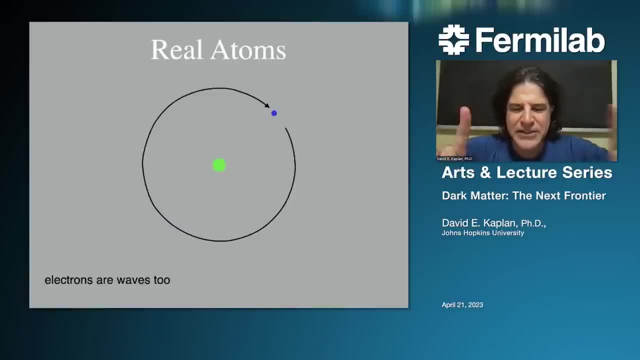 It also turns out that you can do the same kind of two-slit experiments with electrons. You use crystals, but you basically do the same thing And electrons behave exactly in that same photon-like way. They behave like waves. In fact, real atoms are. 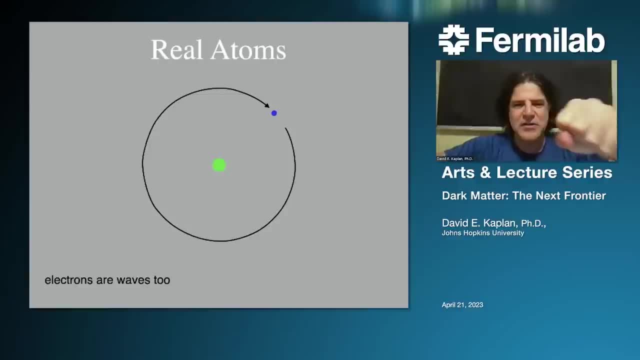 not the cartoon that we all learned when we were kids. There's a proton and some electron going around it. That is not what's happening. The electron really is a wave in its lowest wave state, when it's in the lowest energy state, and the chemistry will call those clouds or shells. 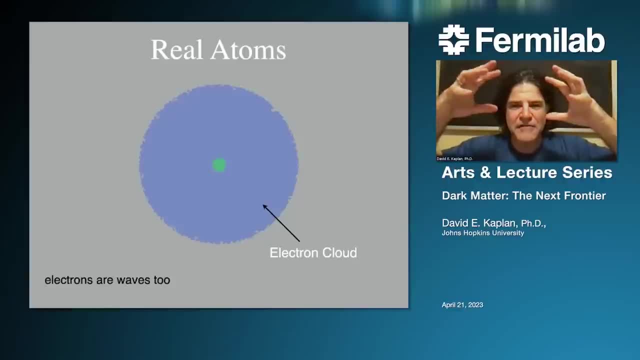 And you should just think of this as this internally fluctuating wave that is stuck in this attractive well, that is the proton. You take a glass of water and you sort of hit it on the ground or on a table. then the top of the surface of water is fluctuating up and down and it's confined. 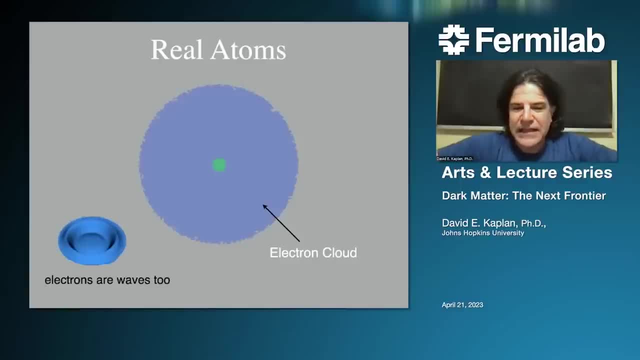 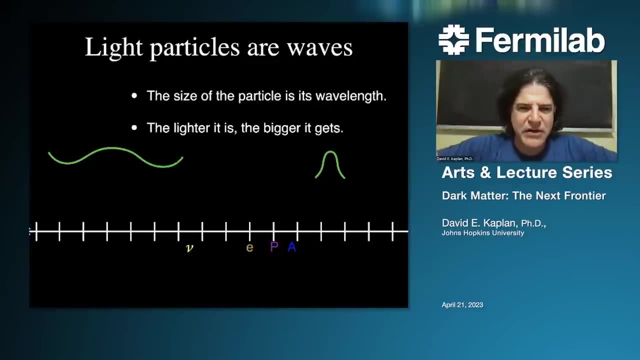 because of the forces of the glass to that space, And that's a much better analogy to what an electron is. It's a wave. The size of the wave depends on the energy and the mass, And so that's why, when we talk about very light dark matter, we actually have to talk. 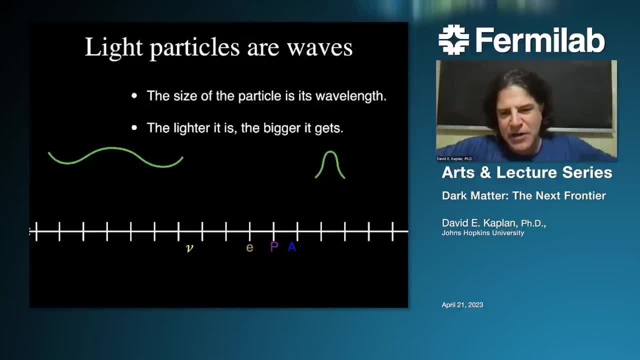 about its wave-like nature. The lighter the dark matter gets, the more like a wave it behaves in the galaxy, And therefore, in order to think about very light dark matter, we have to imagine a fluid of dark matter waves that are either attached to our galaxy or are roaming. 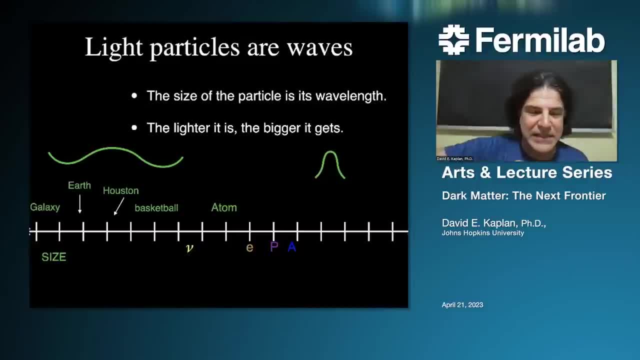 in the universe And as you get to lighter and lighter masses, you really can get wave-like dark matter which is macroscopic. you know the size of, let's say, a ball or a planet or even the galaxy. In fact, since we know that dark matter fits in the galaxy, there is some lower limit. 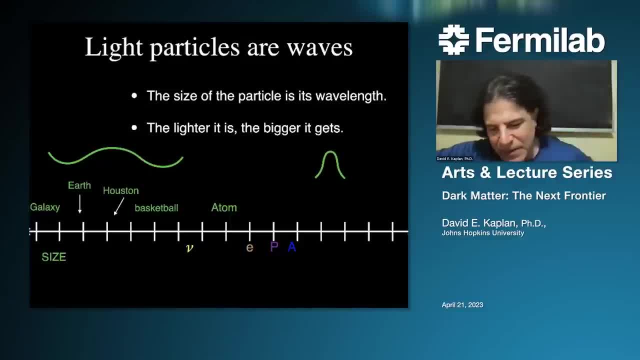 The dark matter cannot be lighter than some particular mass, And it turns out that that mass is roughly 10 to the 28th percentile of the galaxy, And that's a lot of energy. So it's extremely light, but at least there's a limit. It sort of puts a wall below which we don't. 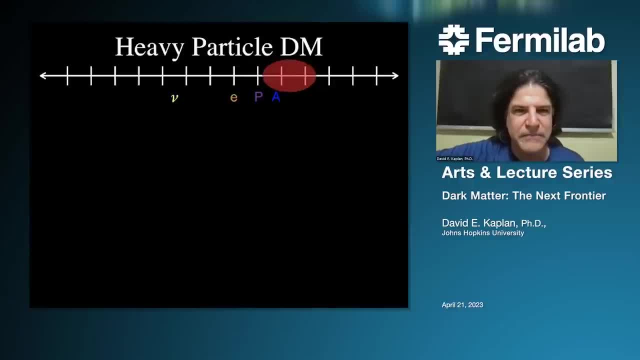 have to really check if we're trying to find the dark matter. Before I go on- maybe, Tom, do you want to- is there like a particular question you think may be relevant now, or should we save them to the end? I know we have finite time. 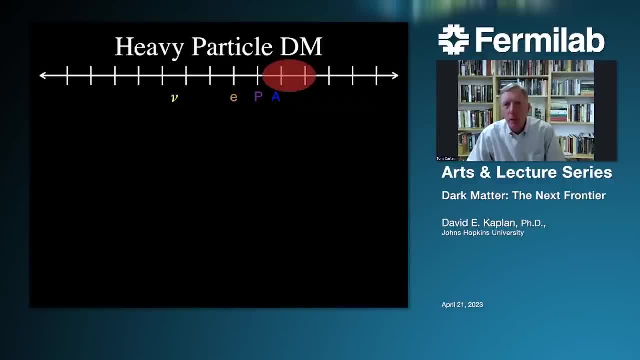 No, I think, I think we're, I think we're good. Some people ask is: is there dark matter here in the, in the solar system, or is it only far away? Does it? does dark matter somehow affect the orbits of? 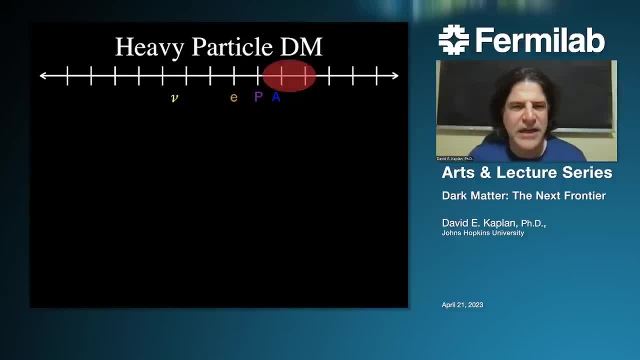 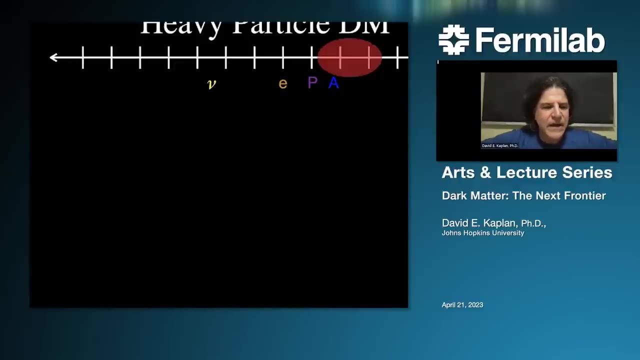 our planets, No great question. So I'll just say one thing about that. One is that, depending on, we know roughly what the density of dark matter should be to explain how our galaxy works. And if dark matter is made of a gas of particles, then yes, dark matter is right here flowing. 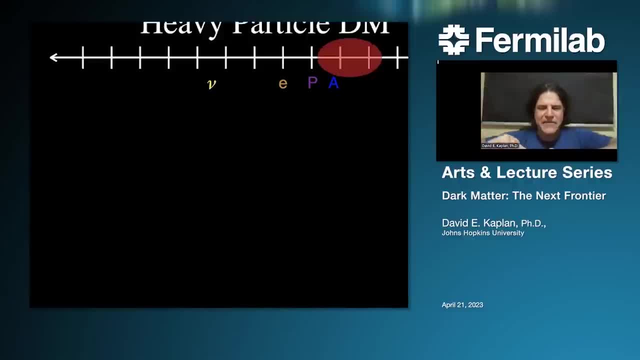 through us. If dark matter is made of very heavy, lumpy objects, then it could be distant objects that are floating around the galaxy, But for most of this particle description, it is flowing through the earth. If this particle gas of dark matter is around it's, it's going to be flowing around. 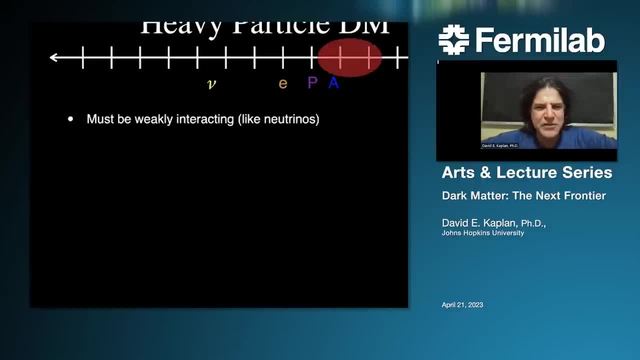 it should be weakly interacting, kind of like neutrinos are weakly interacting. It should scatter very rarely and it should not interact with light. It also should be moving slowly, And what I mean by slowly, which might not sound very slow, but much slower than the speed of. 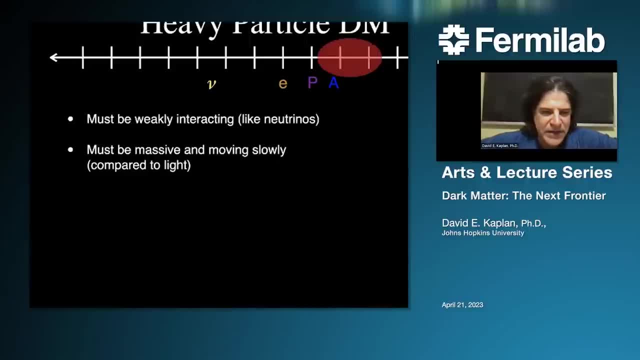 light That allows the dark matter to clump and to create the galaxies and structures. So, because it should be weakly interacting, it should be a massive particle. We coined the term WIMPs For weakly interacting massive particles And the way you would see a WIMP is that if it interacts, 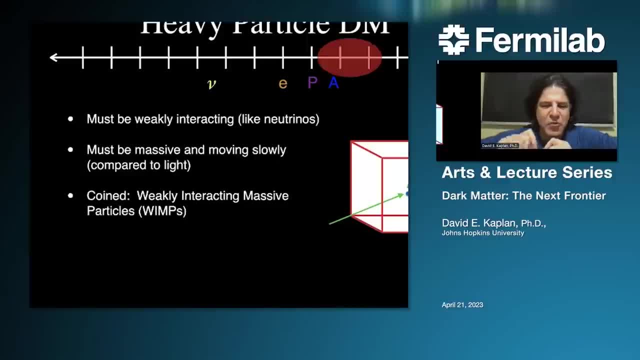 with us, even if it's just very rarely the way neutrinos very rarely interact with us. you have a very sensitive detector, Let's say a liquid or a solid dark matter particle goes in and every once in a while a dark matter particle hits a nucleus in the detector, causes it to recoil and emits. 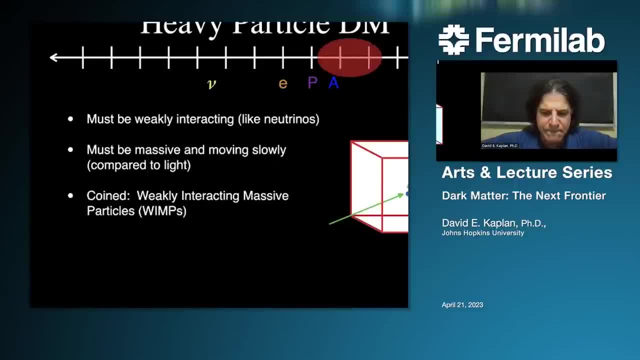 either light, vibrations and or ionizes, electrons, which we can collect. So these are the sort of WIMP detectors Problem. the challenge with it is that even regular matter has trace radioactivity which can send neutrons or alpha particles into your detector. So you should be able to. 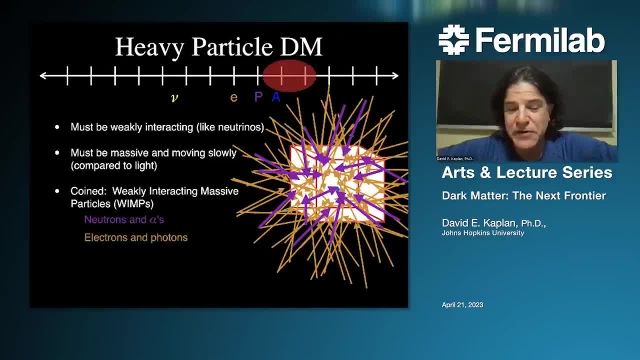 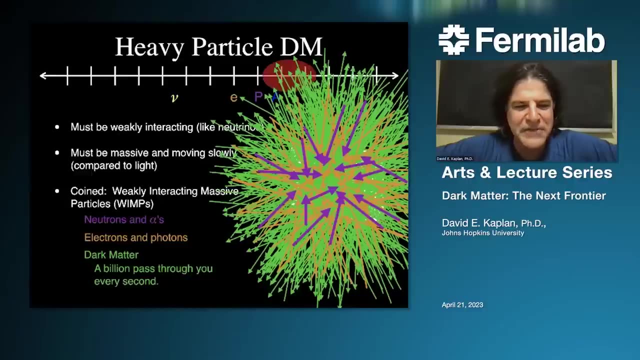 distinguish those two. There's also electrons and photons that are emitted by beta decay, also kind of radioactivity Or gammas, And luckily, though, if the dark matter density is what we think it is, there's an insane number of dark matter particles passing through the experiment every second, And 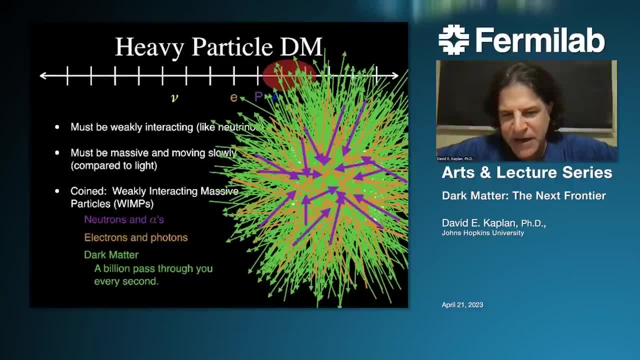 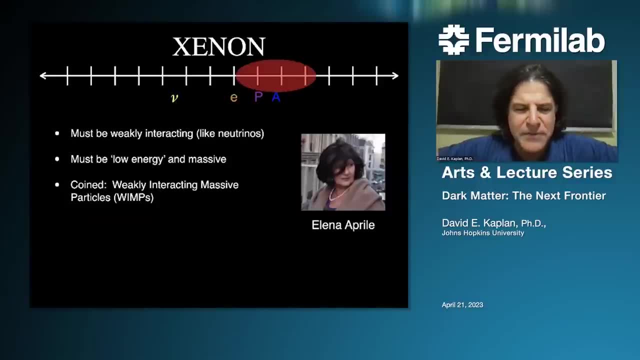 therefore, even for extremely weakly coupled dark matter, there's a hope to see it in this mass range, Let's say heavier than the electron, up to about a thousand times the mass of the proton. So, Elena Aprile, who's a professor of physics at Columbia, she 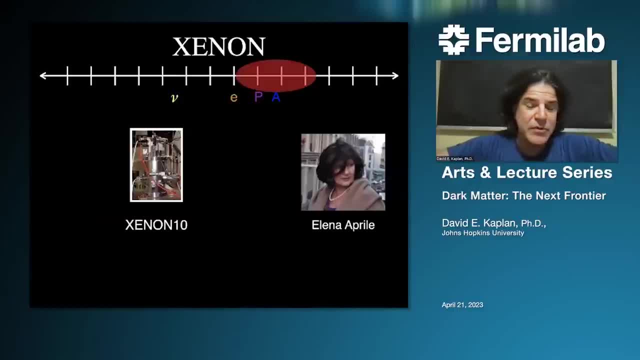 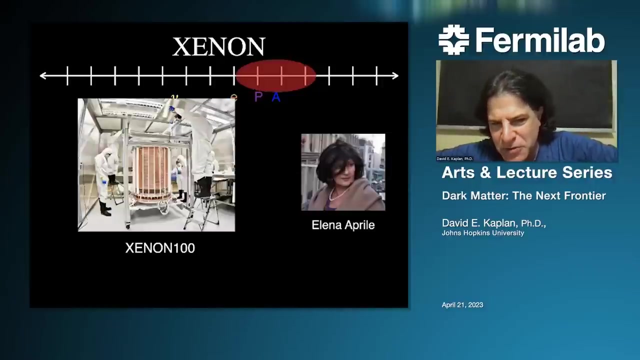 started the path using liquid xenon, which is a nice inert atom gas, but she put it in added liquid form. Xenon 10 was a 10 kilogram tank of liquid xenon looking for this recoil and scintillation light plus release of some electrons. She didn't see it with 10 kilograms, So to see more sensitivity. 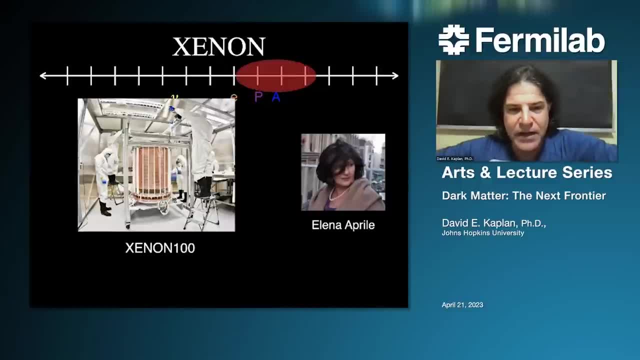 she at the grand Sasso mine in Italy and her group developed a 100-kilogram xenon detector. They ran this detector for some number of years, looked for these effects and could rule out a class of dark matter, because they didn't see it on this mass range. 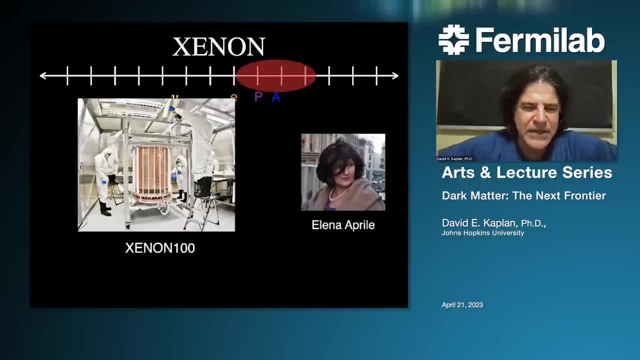 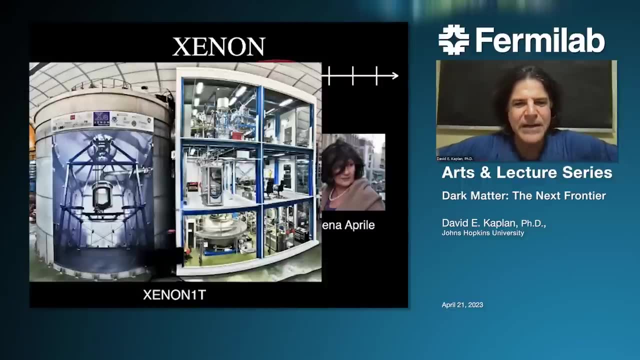 down to a certain weakness of coupling, But not dismayed. they built a one-ton xenon detector in the same lab or in the same mine and they looked and took data for a number of years and didn't see dark matter. And they put another, even stronger constraint. 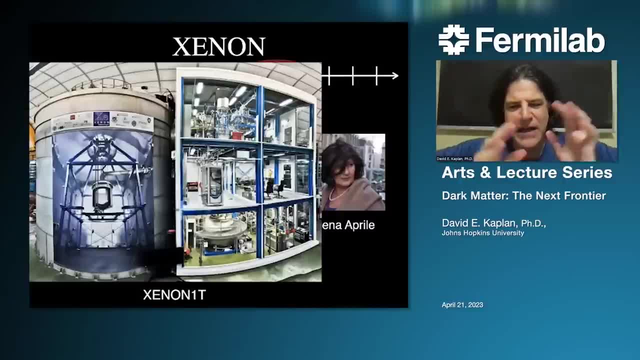 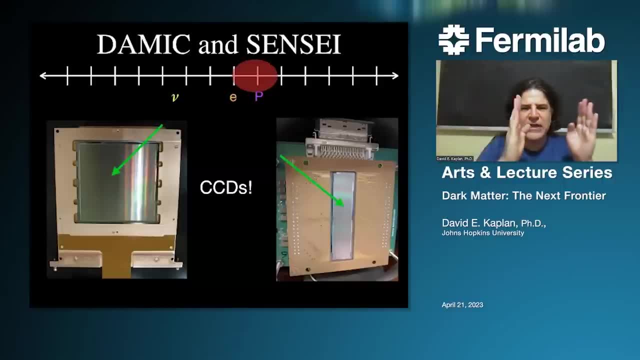 on this range of masses for dark matter and this type of interaction strength. If you want to do somewhat lighter dark matter, there are another class of experiments that have emerged over the last 10 years. In fact, they use at sort of its core basic technology. 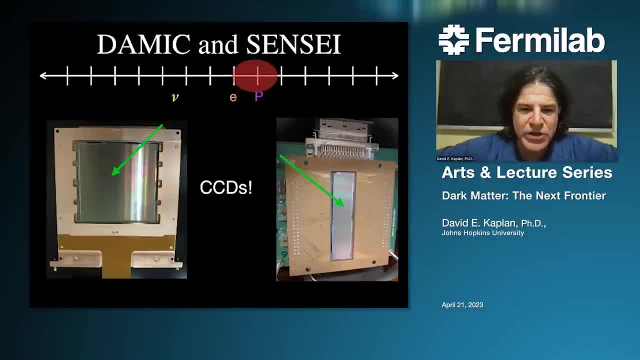 to. These are CCDs, which are the silicon and electrified surface that you have in just digital cameras and your phone, And those will respond to things passing through, say dark matter, particle passing through, kicking an electron and creating tiny currents. And they have fancier versions of these for dark matter. 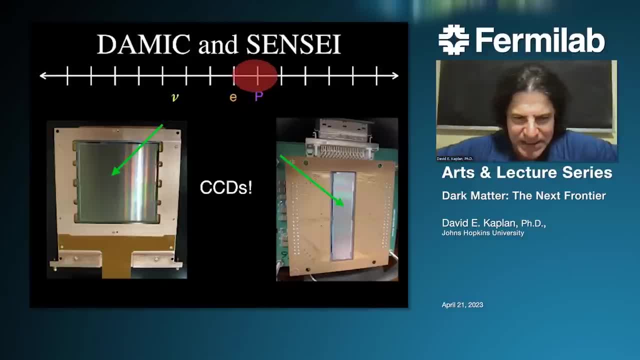 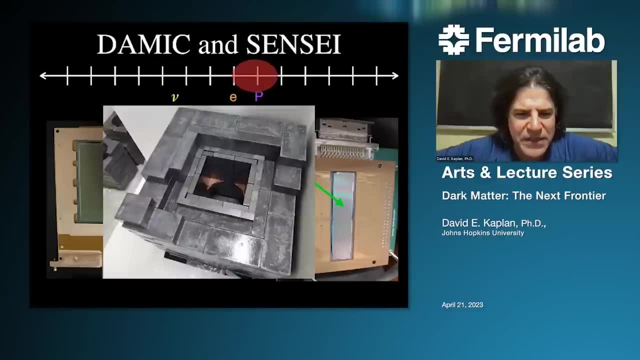 but it's coming out of technology that Already exists, And there are small-scale experiments doing exactly this kind of thing. What's cool about a number of these experiments- this in particular- is that the CCDs- you're trying to block out lots of other things. 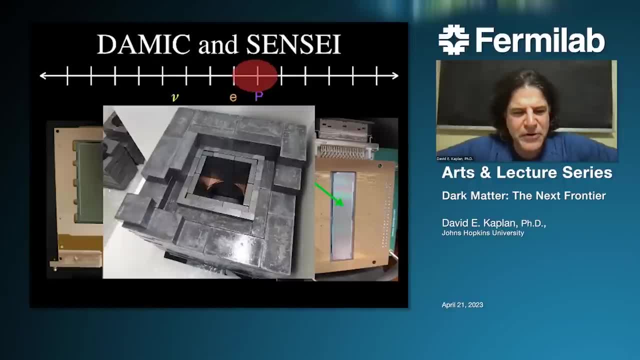 cosmic rays, radioactivity and stuff like that. And so people use lead, but they have to use a very special kind of Roman, ancient Roman lead bricks. And that's because the ancient Roman lead is something that was purified, say, a thousand years ago. 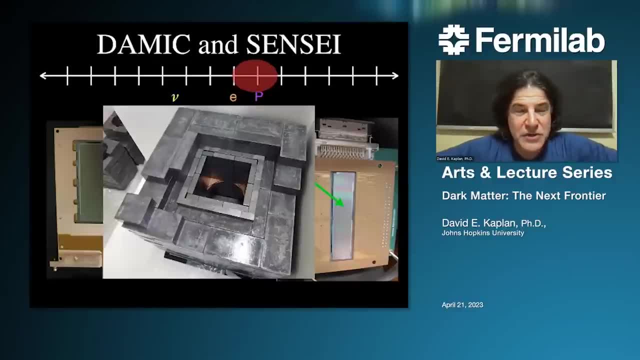 And the trace radioactivity, which was lead 210, that they couldn't. that impurity they couldn't get out because it was a form of lead had enough time to decay over a thousand years, since its half-life was 22 years. 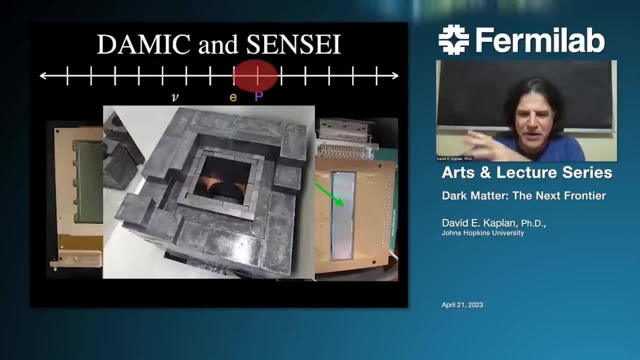 If you use thousand-year-old lead- and it wasn't bombarded with anything else- you do better. So there's a sort of There's a sort of tangle between the physics community and the people doing anthropology or studying the history of civilization. 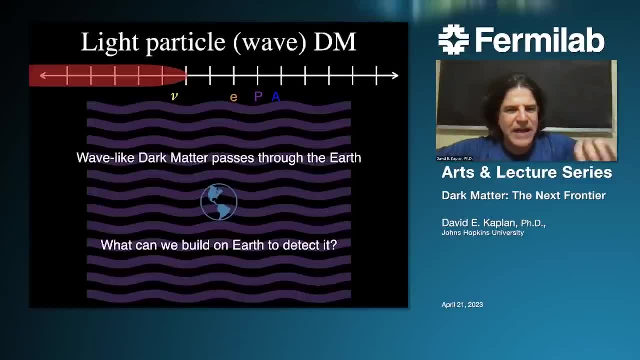 If dark matter is light, so over to the left there, then it is very wave-like. And if there's a wave-like dark matter passing through the earth, you could ask: how could we see it? How would we optimize experiments to try to see waves? 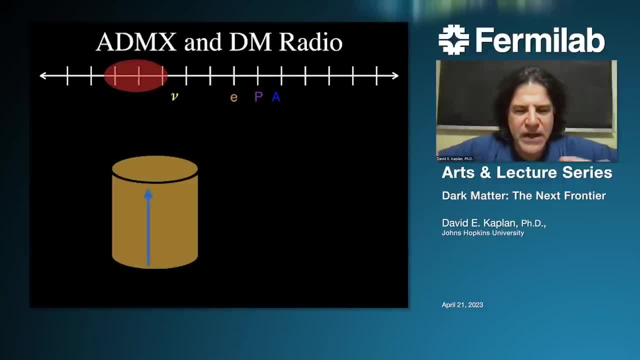 And there's a beautiful, very powerful set of experiments, This one, these are called ADMX or DM radio, But these experiments use the fact that as the dark matter passes through a cavity, it could have some tiny, tiny coupling to light. 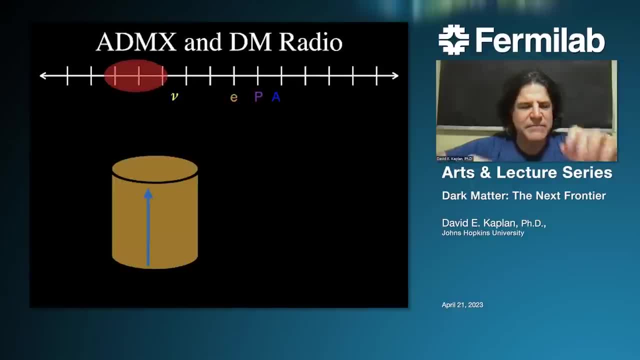 Very weak, too weak to ever affect anything in the universe, But even super weak couplings, if you have the nice, perfect experiment for it, you could get transitions from dark matter into light. For some types of dark matter it's called an axion. you just turn on a magnetic field. 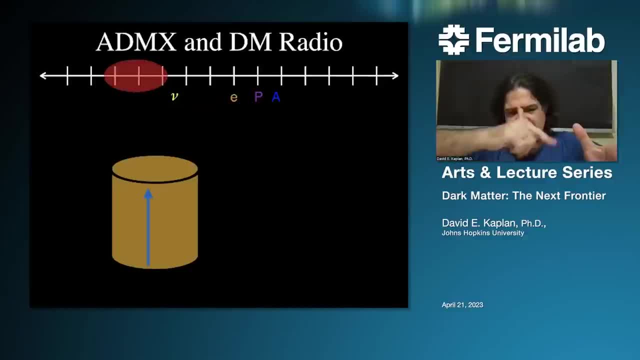 and you will find dark matter if its resonant frequency, which is proportional to its mass, is one of the resonant frequencies of this cavity, an electromagnetic cavity. So axion particles are a type of like dark matter particles, but they really label any. 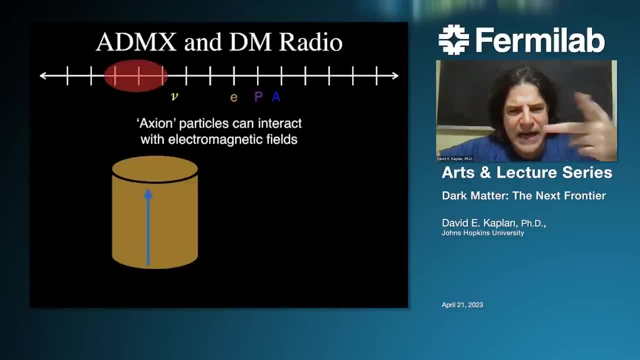 light type of particle that could be dark matter and has some kind of, even tiny, interaction with electromagnetic fields. So you turn on a magnetic field, a wave will come through. it will convert from a dark matter wave to a little bit of an electromagnetic wave. 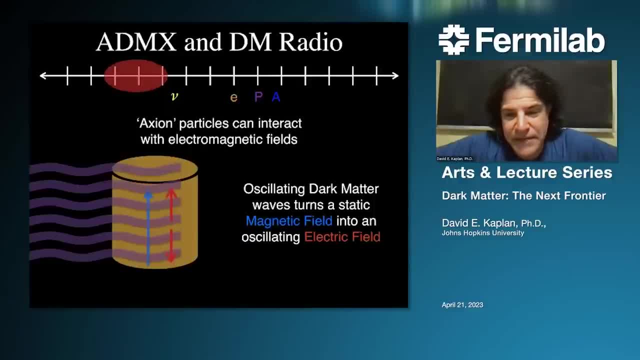 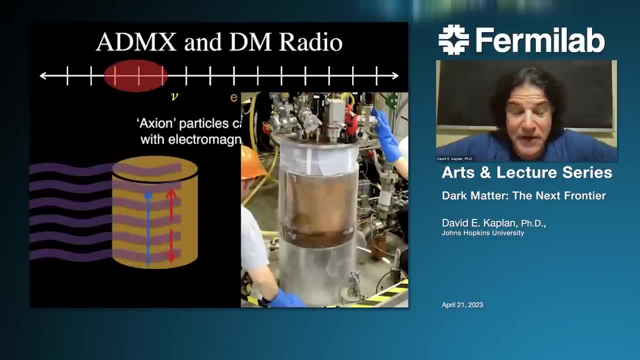 which is a photon or light, And this is the ADMX experiment. It's very hard. You have to make it incredibly cold using cryogenic technology. You put it underground so that it's well shielded and they look for these electromagnetic effects. 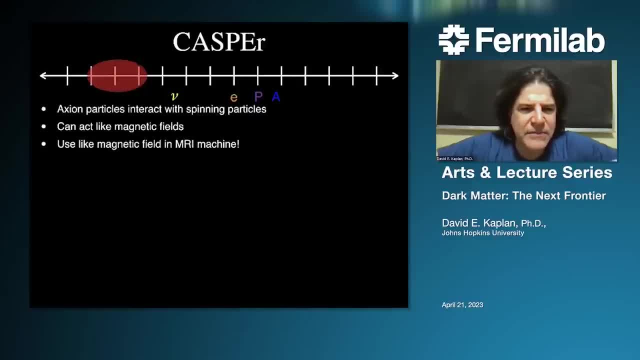 You can also use the fact that particles like this, instead of interacting very weakly with light, they could interact very weakly with matter like the electron And often particles like this. the simplest theories are that they're not very weak, And so you can use these particles to 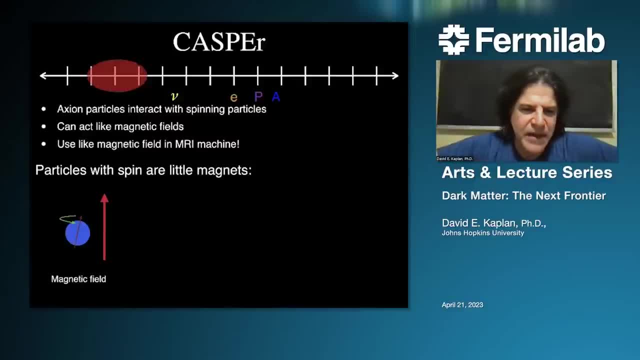 interact with the spin of the electron, And particles with spin like the electron are like tiny little magnets. They have magnetic dipole moments And when you put a little magnet in a magnetic field, even if it's tilted a little bit, it will process around the magnetic field. 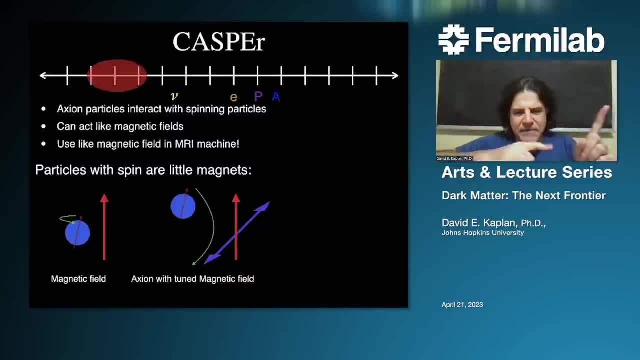 And if you turn on the axion field- since the axion is some kind of wave that's oscillating back and forth- That fluctuation can cause these little electrons to flip. This is exactly it turns out how an MRI machine works. 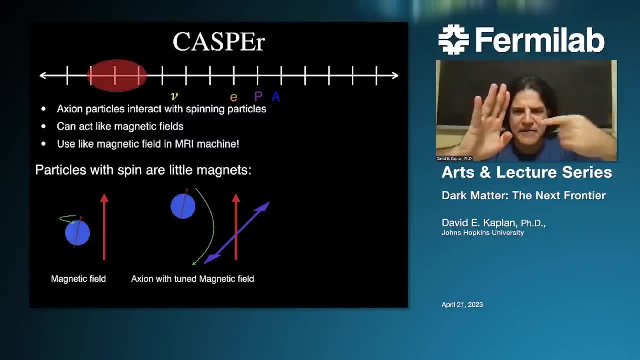 You put in a big magnetic field a tiny fluctuating magnetic field and you can learn about the density and the properties of the matter that you're looking at Here. the fluctuating field is not something we turn on. It's something that could be the dark matter moving through the experiment. 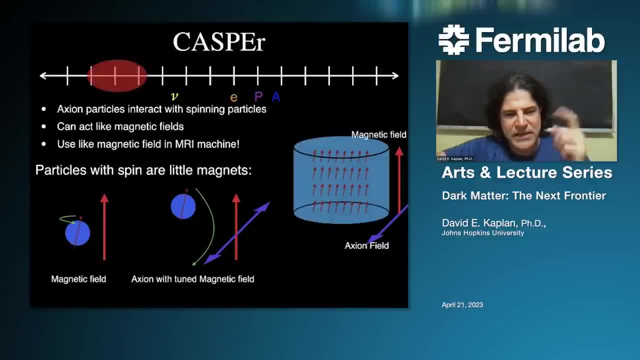 And if you flip the little spins- since all those little electrons or nucleons, those spins themselves have a little bit of magnetic field- you can use extraordinarily sensitive magnetic detectors, something called a squid loop made of superconducting material, and detect extraordinarily tiny magnetic fields and therefore potentially see these flips. 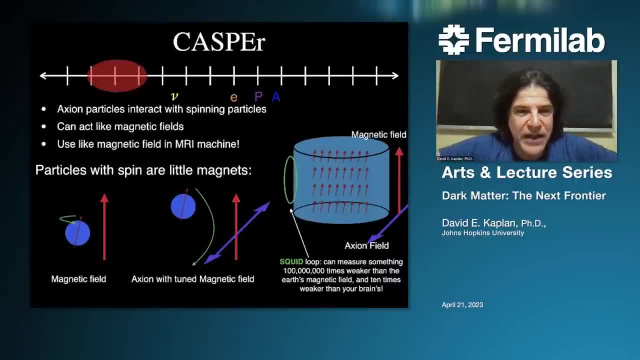 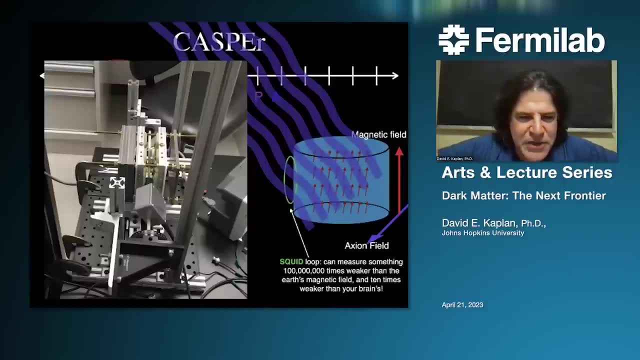 due to a background axion field or some kind of wave Like dark matter wave comes in and there actually, I took a picture of a friend of mine as building such an experiment and this was the prototype and since this was a new type, 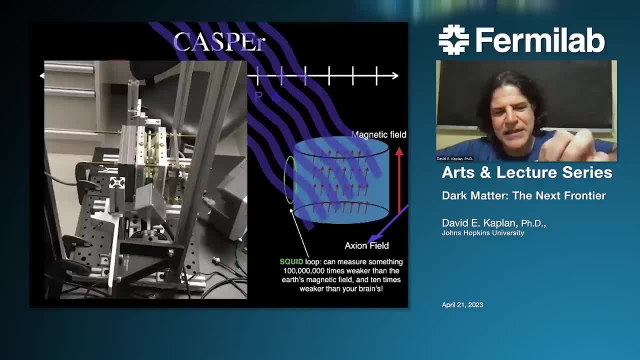 of technology. we weren't at one ton yet. The size of the experiment: this one was about a centimeter cubed, just to prove that technology works. and he is now building the 10 centimeter cubed version where he actually could detect. 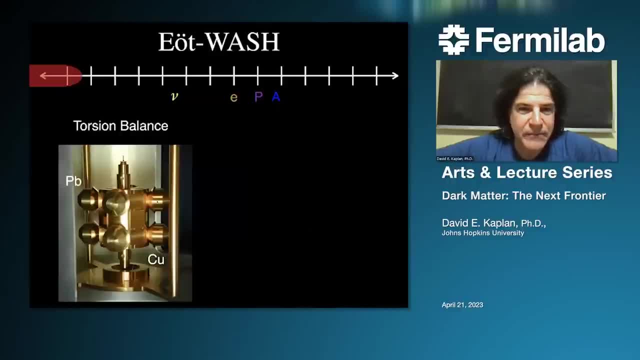 it or see new. So this is a very interesting experiment. The last one I'll talk about is something called torsion balance experiments. If the dark matter wave, is if dark matter is super light, then the wave is very long wavelength and sort of oscillates very slowly. 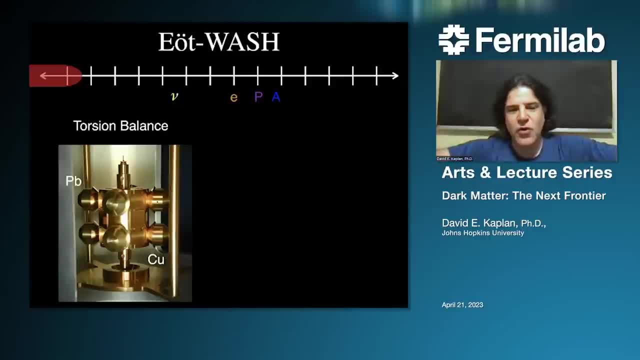 And what you could see potentially is a force on one of these torsion balances, which are used for other purposes. They're used for measuring the properties of the gravitational force of the earth itself. If there were some funny properties, it would cause a torsion balance to spin back and forth. 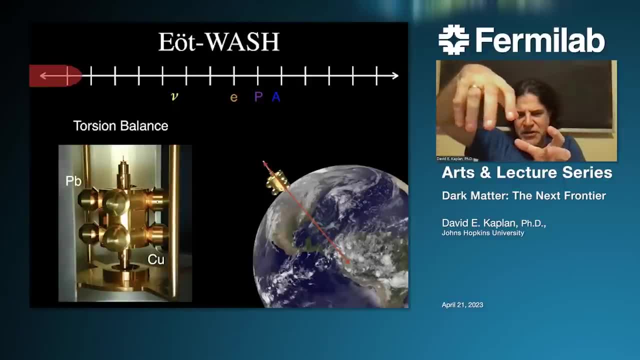 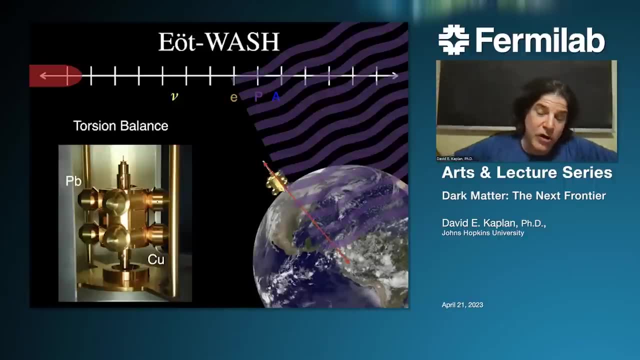 And if you have one of these torsion balance experiments on earth, looking for strange forces towards the center of the earth which could cause spinning, such a balance would also feel the forces due to wave-like dark matter passing through the experiment experiment And it has to do with the property that for the gravitational force, all types of 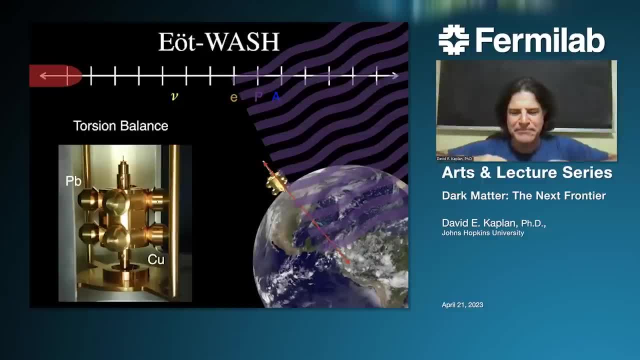 matter fall the same way. That's Galileo's experiment, not really doing this, but dropping things off the Tower of Pisa and everything falling the same way. In the same way, if there's a new force, you can show that new forces will not have that property will violate the so-called 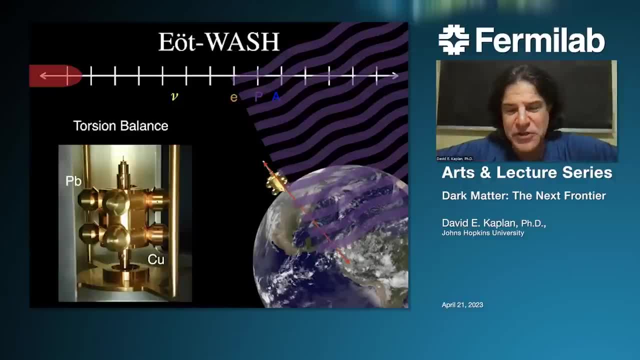 equivalence principle and will put different forces on different types of materials. And so you set up experiments with different types of materials on either side- in this case torsion balance with lead and copper in this one case- and you look for a torque on this balance experiment. 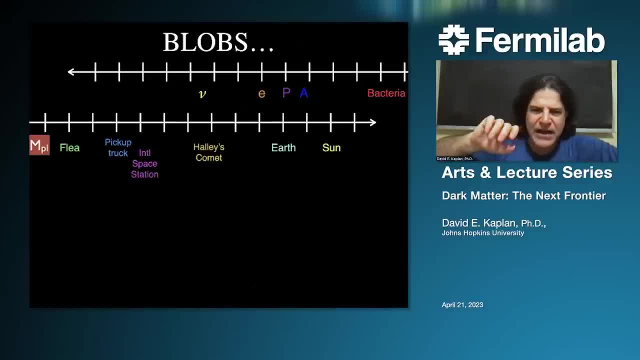 If dark matter gets super heavy, then at some point above a certain energy scale called the Planck scale it cannot be a particle. And that's because a particle that's heavier than the Planck scale, its gravitational force on just the single particle itself would collapse it into a black hole. So particles heavier than 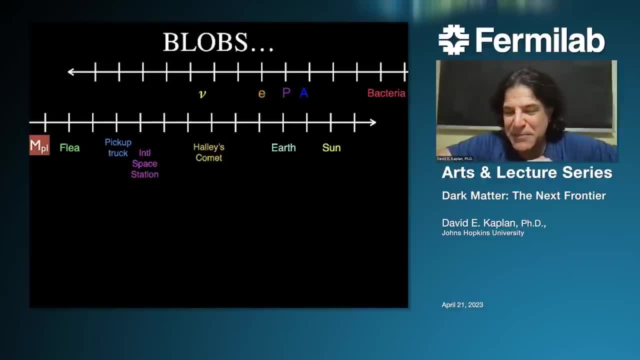 this Planck scale, which is 10 to the 19 times the proton mass, are not particles, they're black holes. But you could have a kind of matter that's made of something other than atoms, but it could come in clumps. Our matter comes in clumps. We have planets, we have stars, So perhaps the 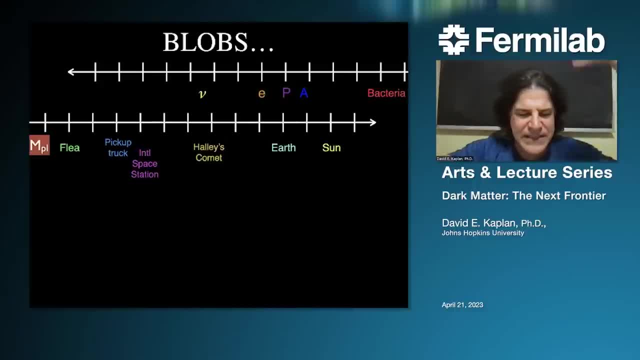 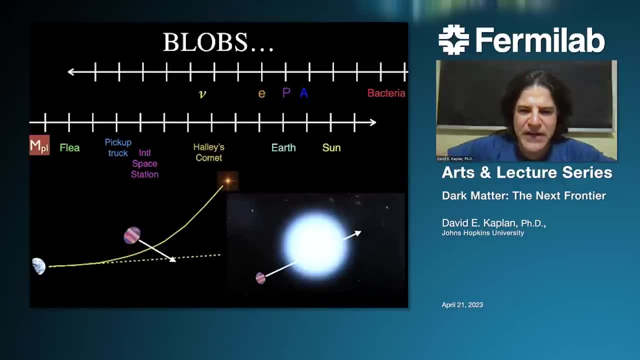 dark matter does as well and is passing around the galaxy in this clump-like form. Well, a very clean way to look for it is if these lumps are moving around the galaxy. you can stare at a distant star and wait for some clump to move nearby its line of sight and you will see a 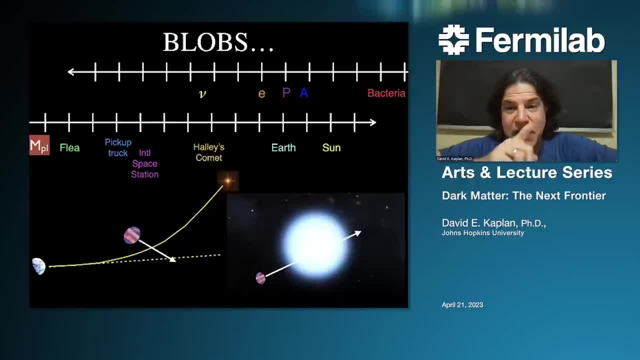 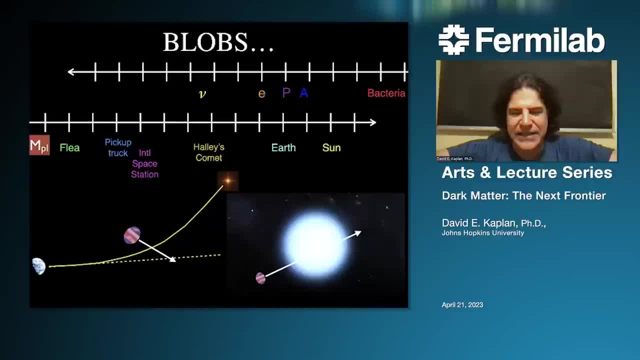 and it can pass near or in front of the star and it changes again due to delicate lensing effects. it changes the brightness of those stars, And so people have looked for dark matter in this way to see if it's made of clumps and it's not for some masses but in other masses they don't. 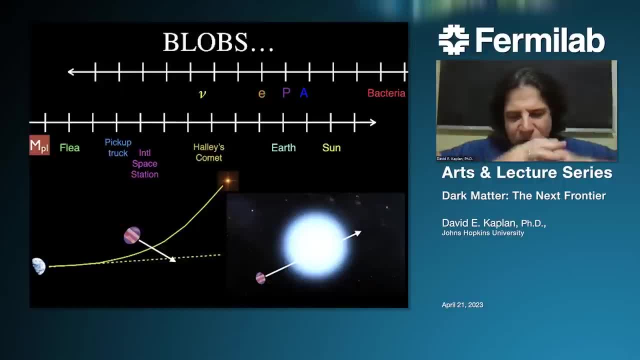 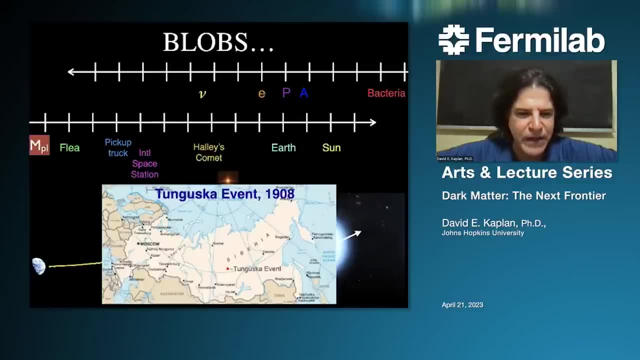 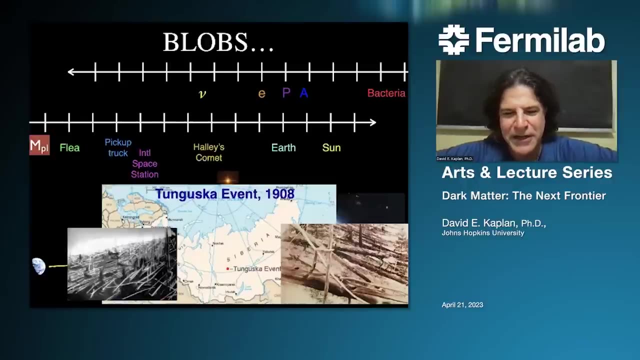 have the sensitivity to tell yet. So this is an ongoing direction that people are looking to potentially see dark matter which is more macroscopic. Some people think that the this famous event in 1908 was some dark matter clump hitting the earth and causing some of this.